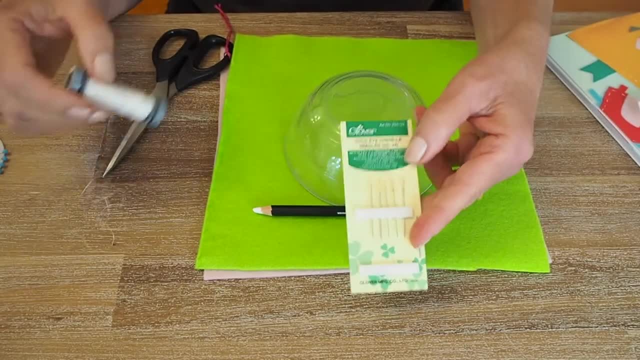 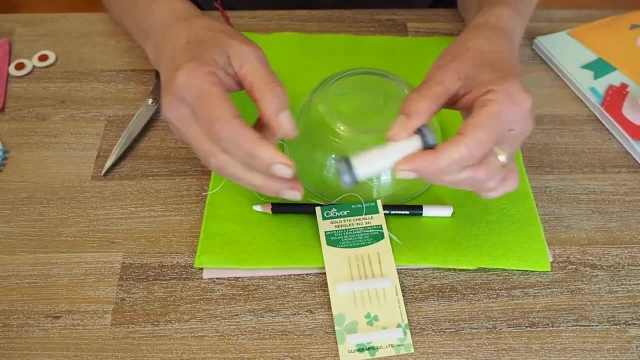 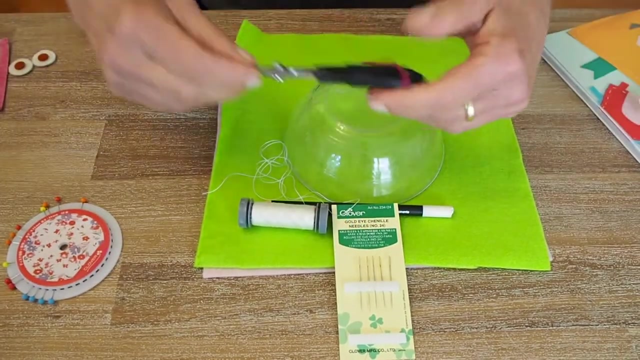 I'm going to need a pair of silver chenille 24s, and I use them because they're nice and small and they're perfect because I use ordinary sewing cotton when I sew my softies, and this one is one by Orifl. you're also going to need some pins, a really good pair of scissors to cut, and 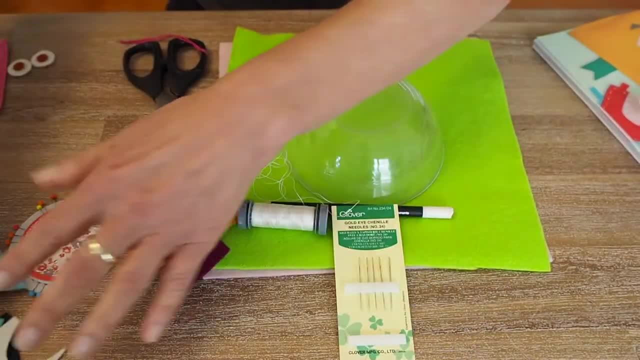 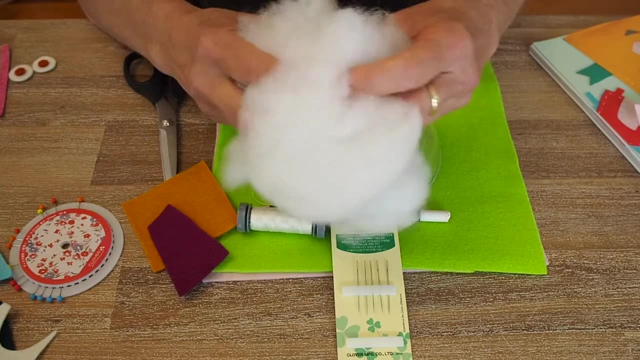 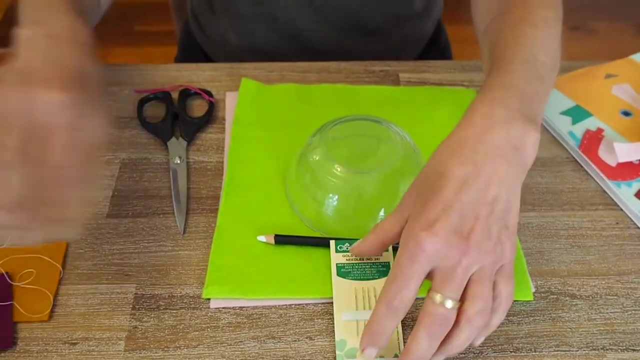 some scraps of felt for the facial features and, of course, I've almost forgotten that the most important thing is the stuffing. So I think we're ready to begin. so let's just move everything out of the way, and the first thing I'm going to do is I've got my two layers of felt here. 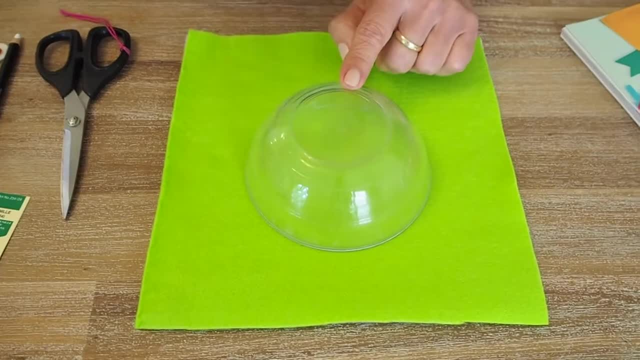 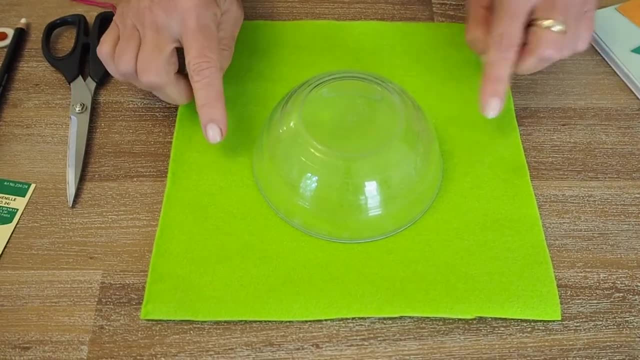 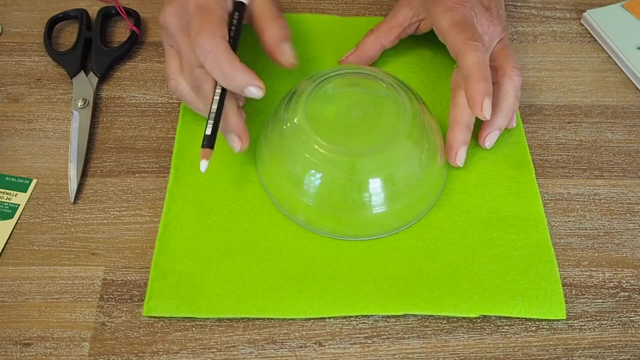 and I'm going to draw my circle, which is the body of Circle Zenki. Now, remember, you want to leave or have a border all around the edges, because these are going to be her arms, legs, hair, whatever you want to add to her. Okay, so let's see. 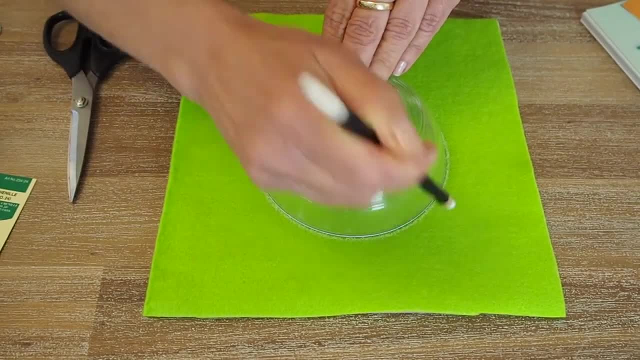 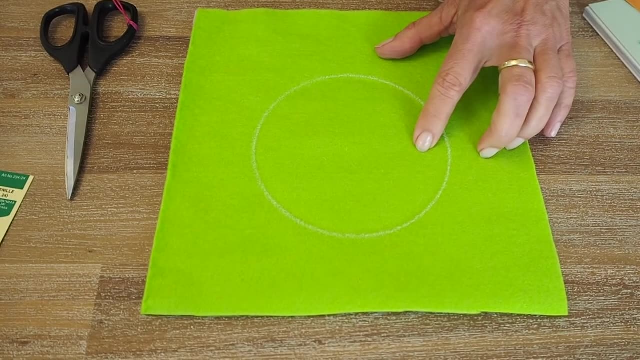 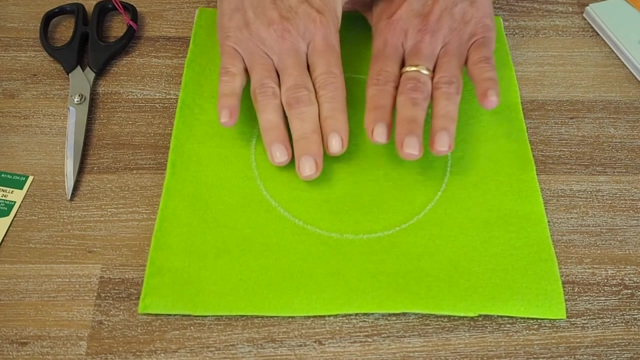 this pencil is great because it actually rubs off easily and it's not quite as messy as a graphite pencil. Okay, now, um, I'm going to. you could at this stage, if you want, to put on any facial features, but I'm going to do that at the ends today, so that what I'm going to do now 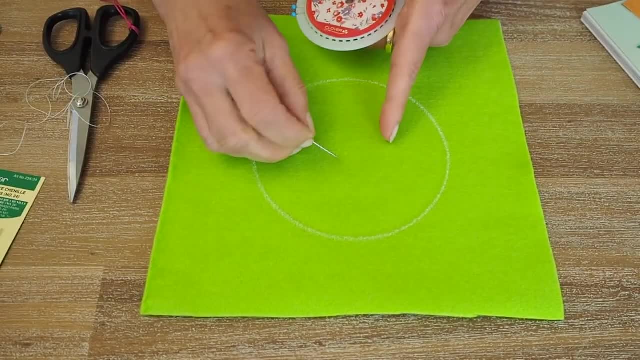 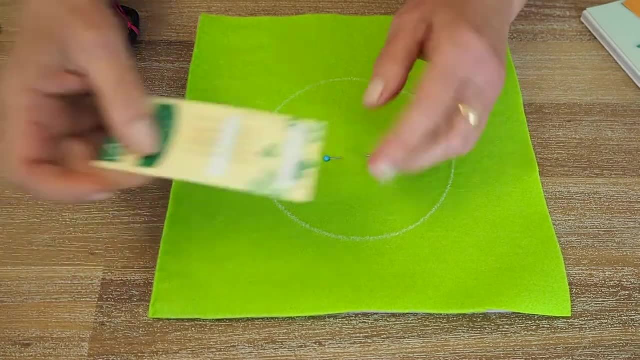 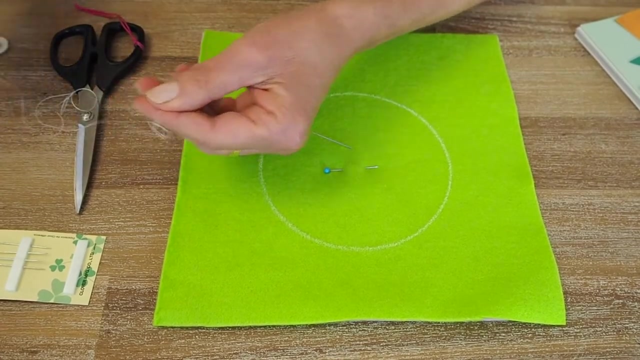 is, firstly, I'm just going to pin the two layers of felt together and then I'm going to thread my needle. So I'm going to take my chenille needle and I'm going to show you how I thread. Okay, so I've got the end of my thread, which I'm going 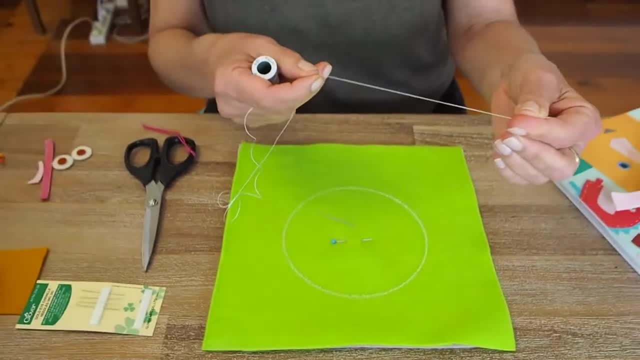 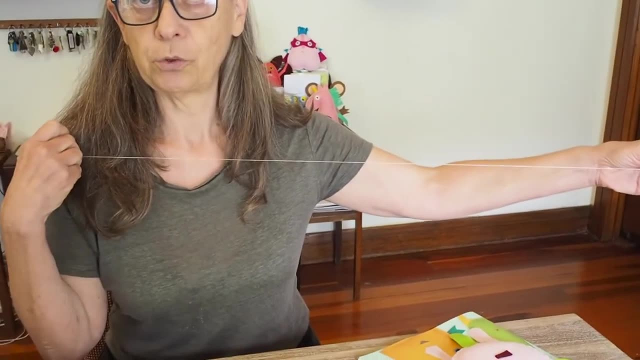 to hold on the fingers and I'm going to show. I'm going to pull the end of the thread, if you can see, and the other end I'm going to take to my chenille. So I'm going to pull it through my shoulders and then I'm going to. 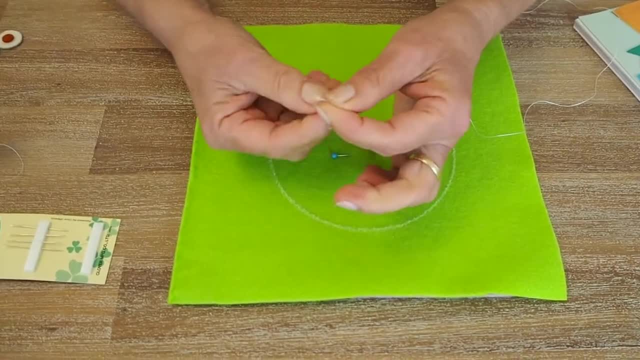 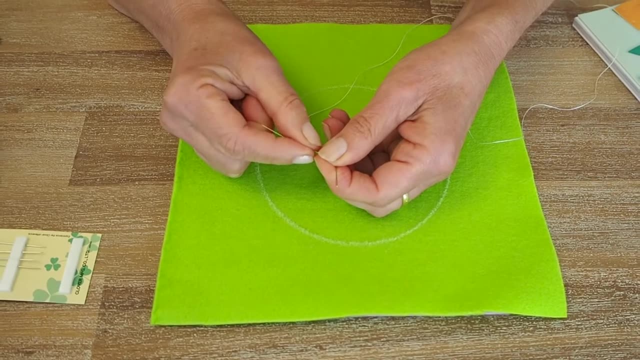 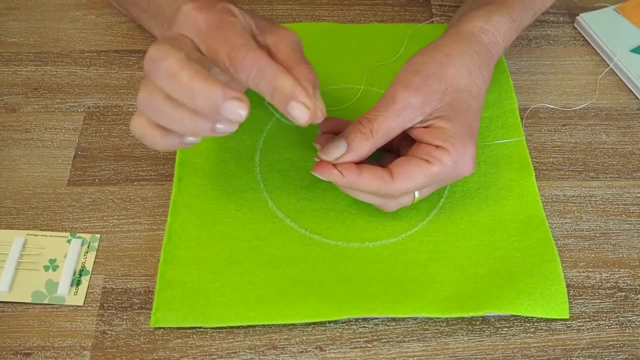 cut. now here is my needle. there are different ways of threading a needle. I'm going to show you today just one of the methods. if you need other ways of threading the needle, you can just go to my other youtube posts. So I've just got a tiny little bit of the end there and I'm going to just put it. 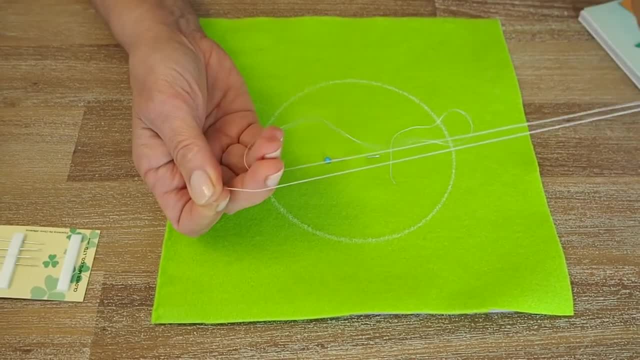 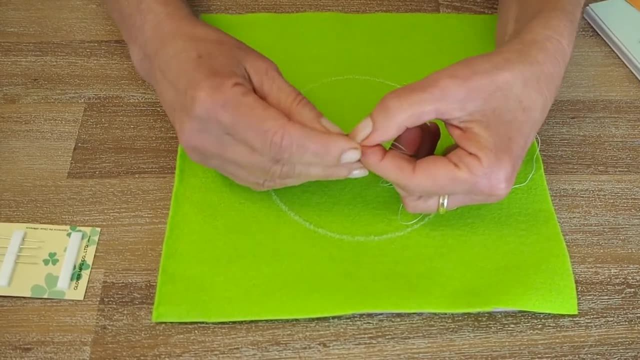 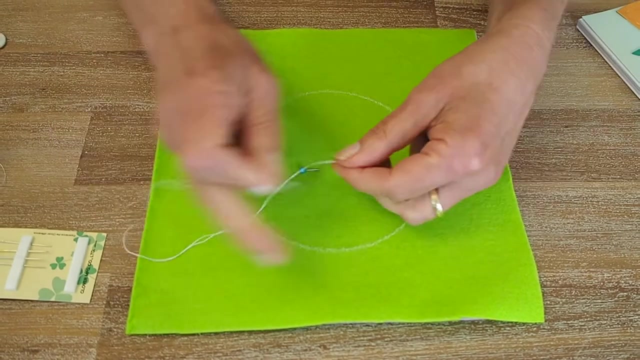 needle. Okay, and now I'm going to bring the two ends of my thread together, and there are different ways of making a knot and, of course, I've got a YouTube tutorial about how to make the knot. Here's just one of quite a fun trick to. 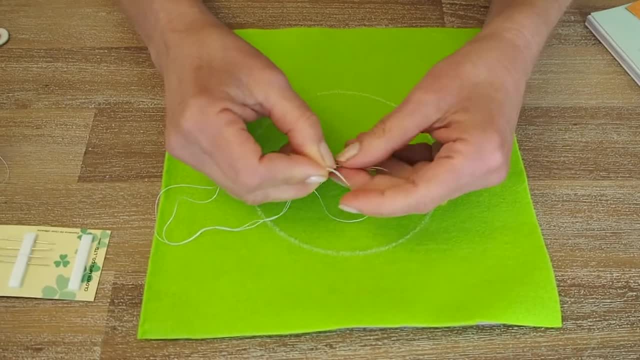 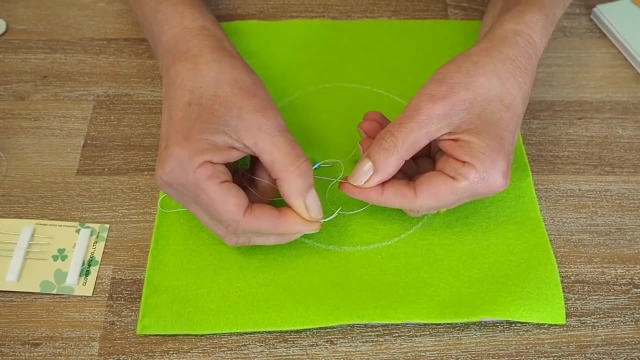 tying a knot. So I'm going to get the eye of the needle. I'm just going to put it on my finger, then my thumb there to hold it. I'm going to get the two ends of the thread and I'm going to put them right next to the eye. 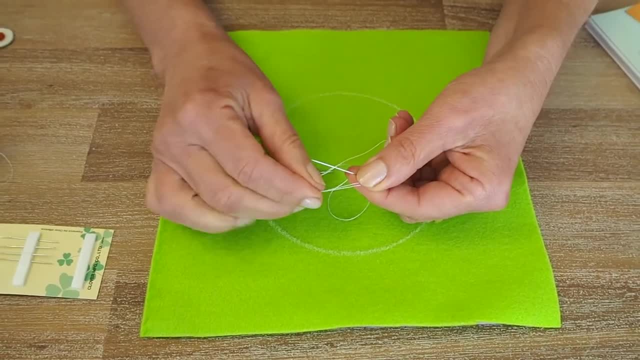 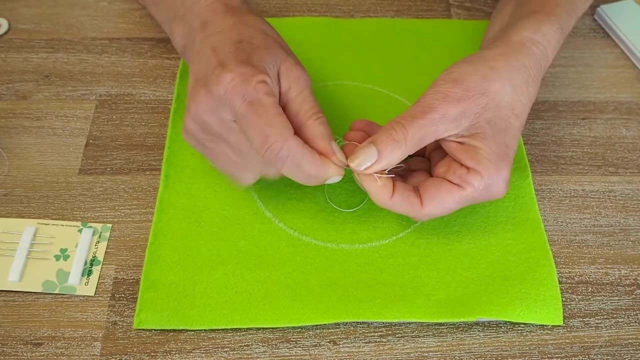 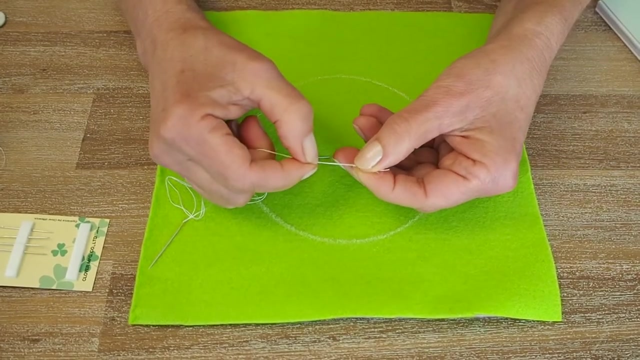 of the needle, put my thumb over it and now I'm just going to do a couple of wraps. let's do one, two, three, let's do four wraps. so, as you can see that I'm going to very gently pull them to the end and hopefully I have a knot- Yes, I do. 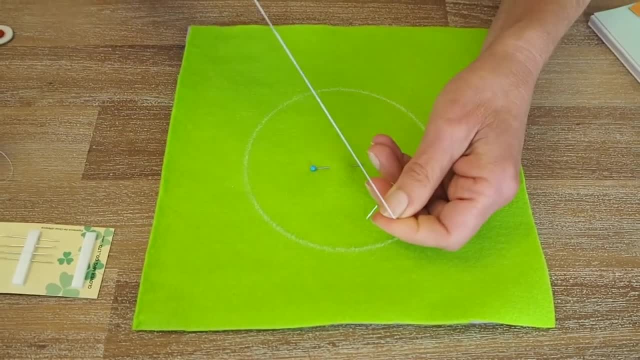 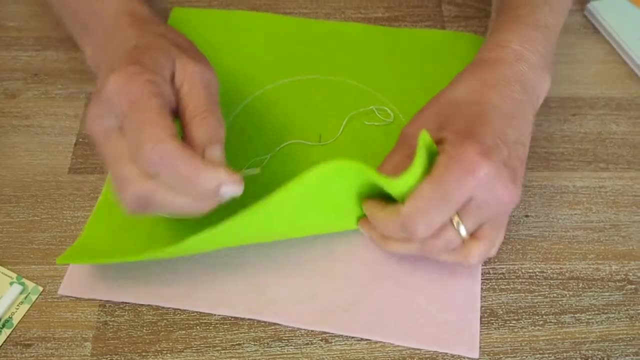 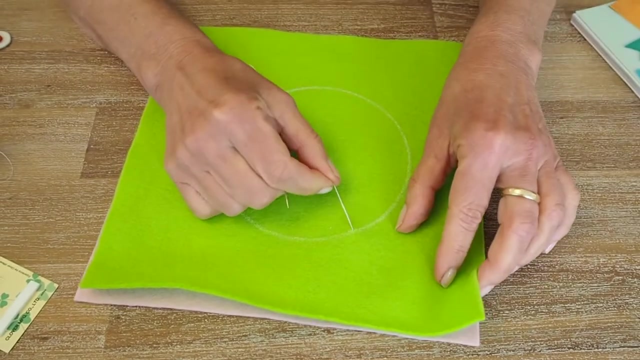 bit of a messy knot, but it's still a knot. Okay, now, let's start the sewing. okay, now, let's start the sewing. now. I'm just going to turn around now, I'm going to start in between the two layers of felt and I'm going to bring the needle up. so there it's, knotted in. 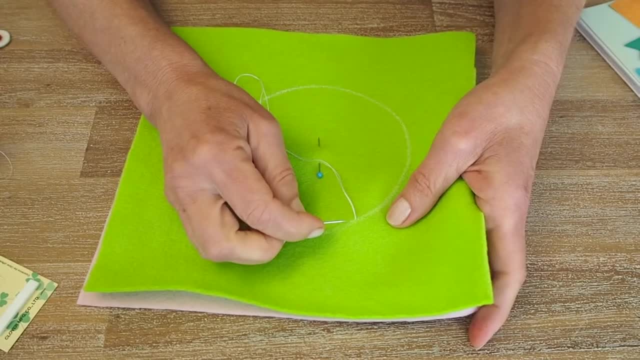 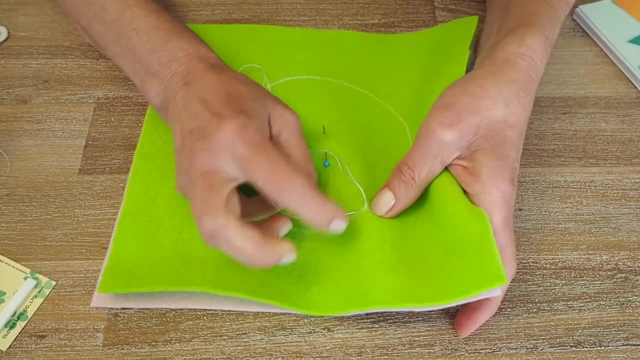 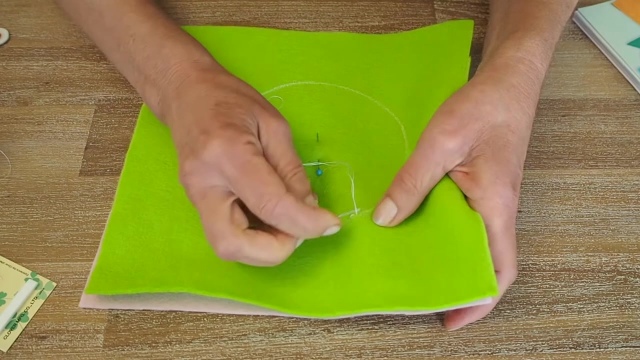 but just to make it really, really secure, I'm going to do a double stitch To do that. I'm just going to go back a little bit and forward and come in more or less the same place you started. and I'm just going to go back a little bit and forward and come in more or less the same place you started and I'm just 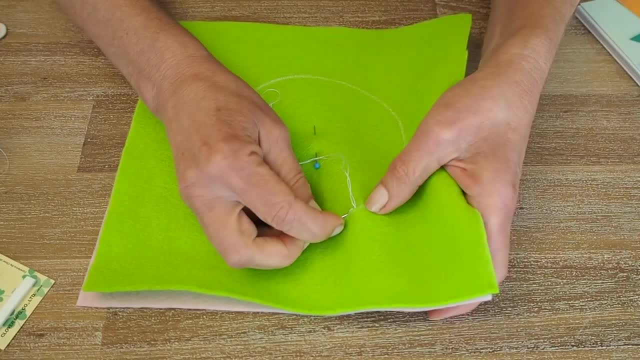 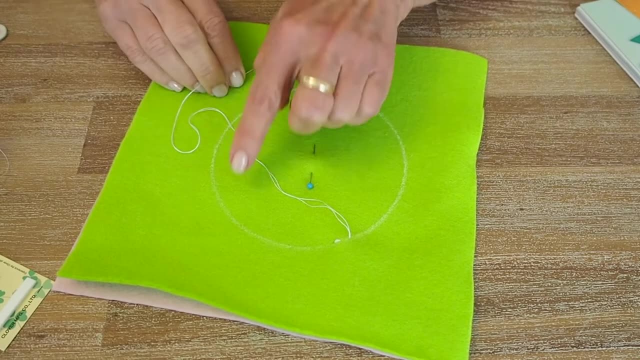 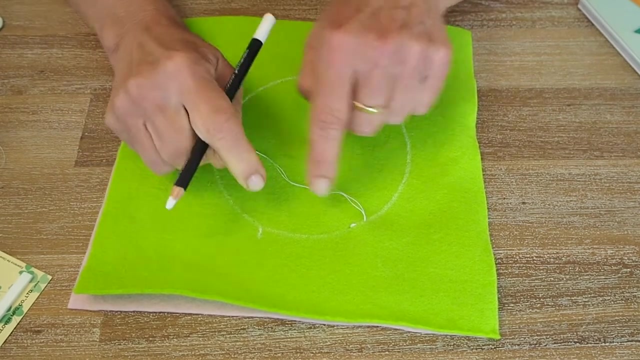 going to go over that one more time just to make sure it's really secure, because you don't want your thread or stitching coming out after all that work. Now I'm going to do a running stitch all the way around until I get to about here, and I often will draw just a little line there so kids know when to stop. So we 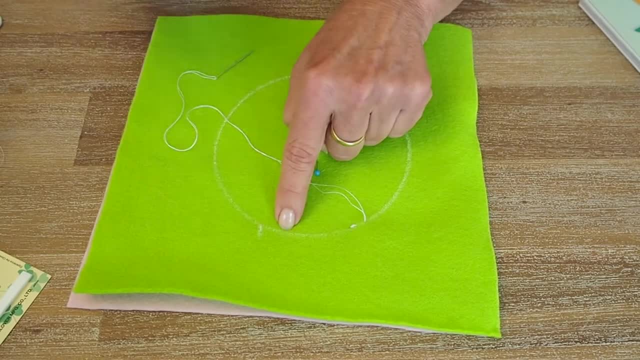 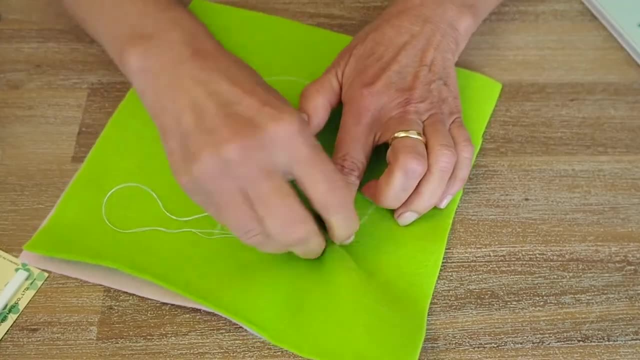 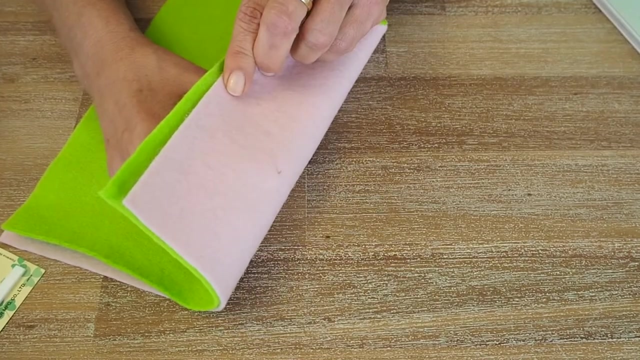 have our stuffing gap here. so how do I do a running stitch? well, it's just basically up, down and up. So how do I do a running stitch? well, it's just basically up, down and up, pull. I don't take my needle to the back because there's no line to see there and I just think. 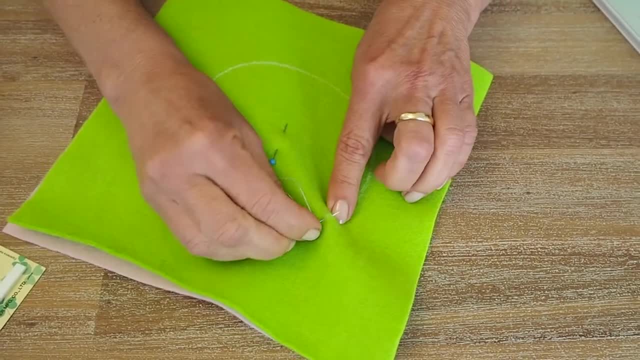 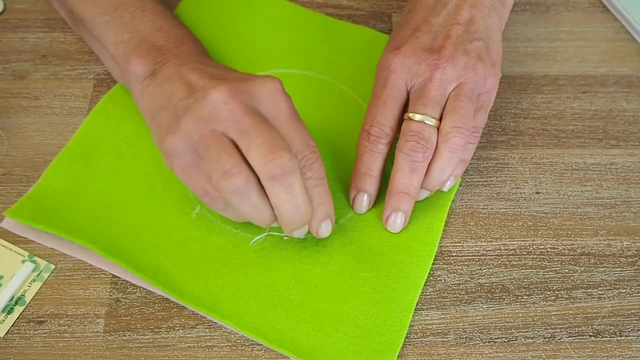 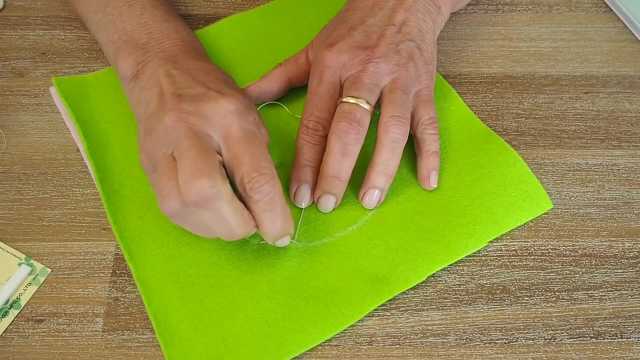 it's easier for kids, so I go down and up, okay sometimes. I just get the kids to feel as soon as that the needle hits the table. they can feel it and gently push up. One of the kids in my classes once told me it should be called a diving stitch, not a running stitch, and I actually agree. 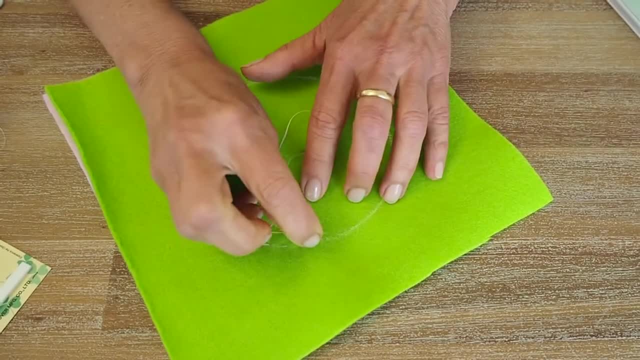 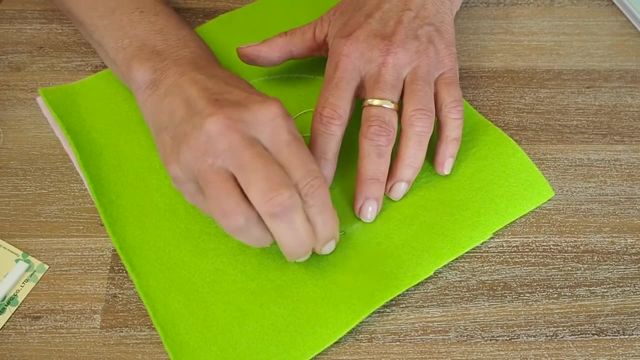 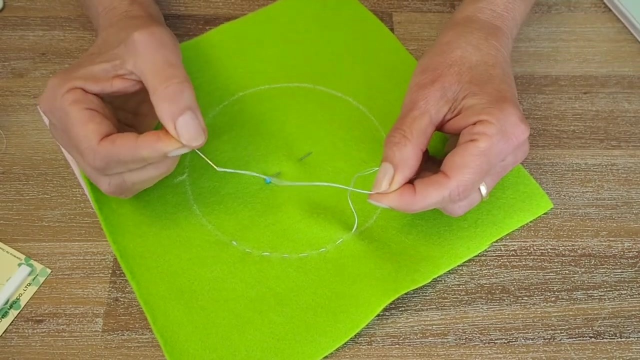 I think that's a much better description of this stitch. So here we go. it's a running stitch, just keep going along the circle. and I always remind the kids- and this is very important when they have about this much thread left, to stop and end their thread, because if they sew right up until 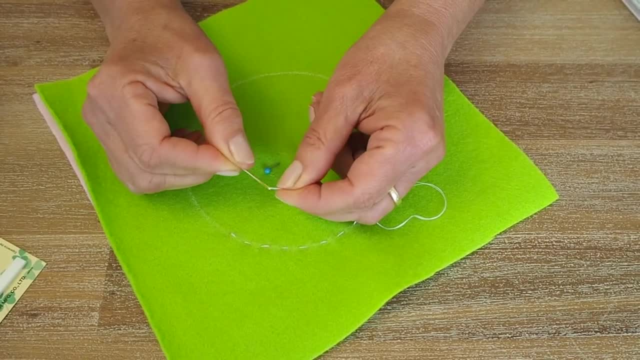 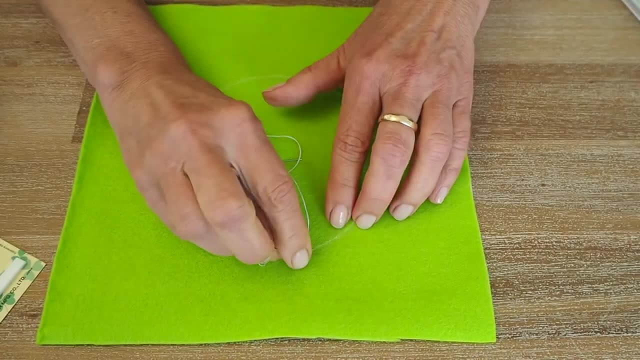 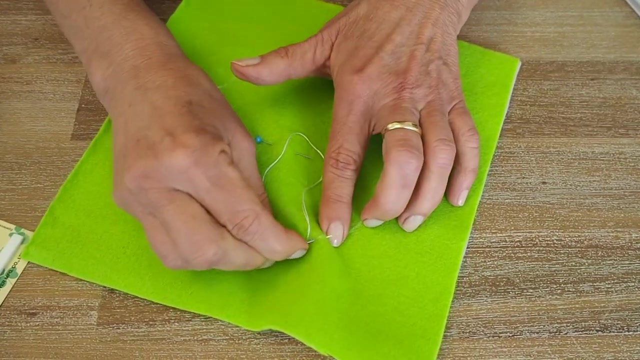 the end where their needle is. it's going to be impossible to end their thread, So I'm just going to keep on going And if you ever have any questions, you can email me or leave a comment below, and I'm always happy to answer questions. 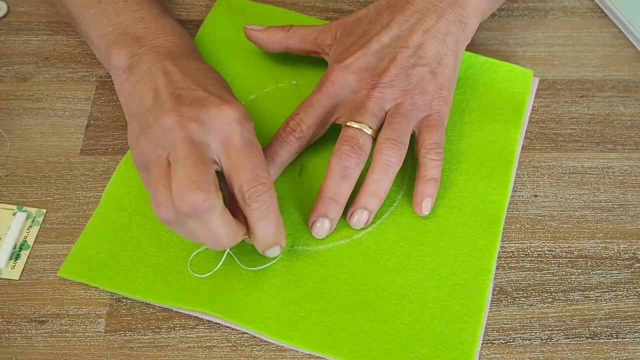 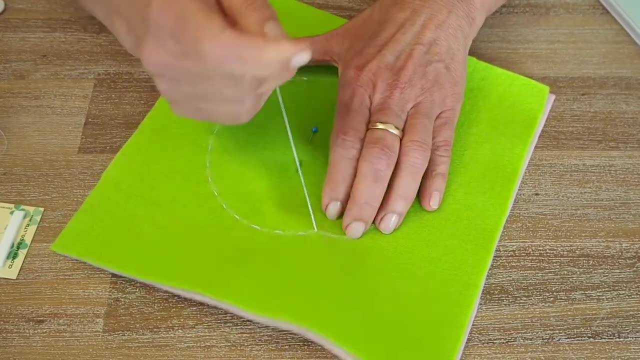 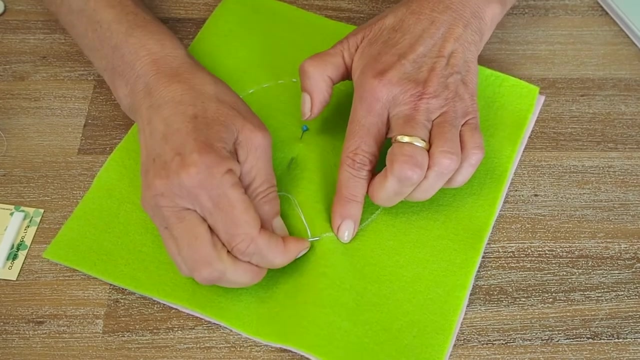 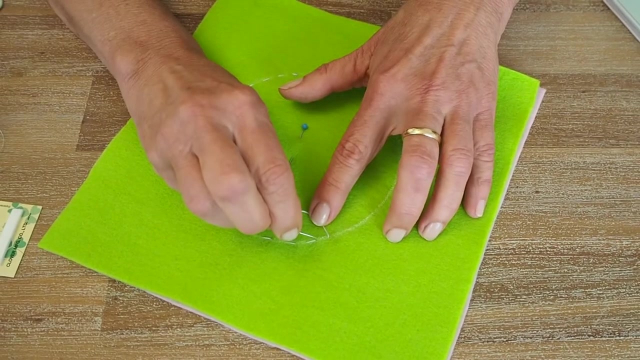 Now, as you can see, I've got, you know, getting to the end of my thread, so I'm going to do one more stitch, and now I'm going to end it. and how do I end it? just the same way that I started, I'm actually. so I'm going to go backwards. actually, I'm going to just do a bigger stitch. 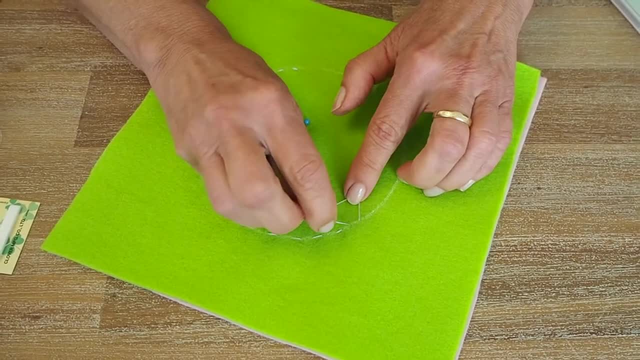 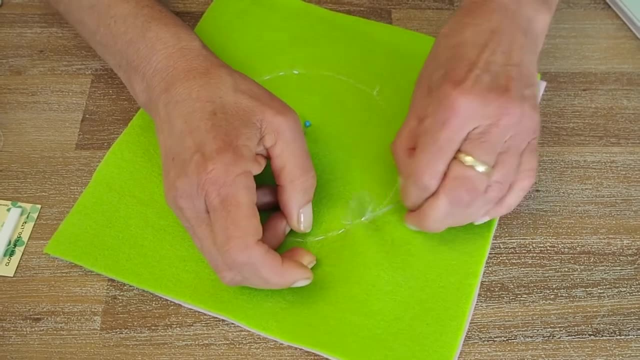 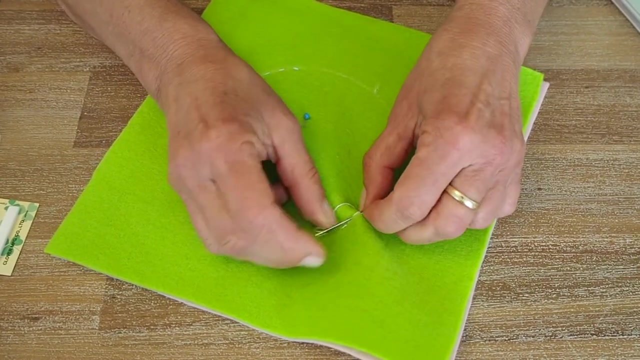 like that. so there's a nice head gap and I'm going to go backwards and forwards into more or less the same place where the thread has come up through the felt and I've got one stitch and I'm going to do the same stitch again. so now you have this little double stitch and now to get rid of the end of the thread. 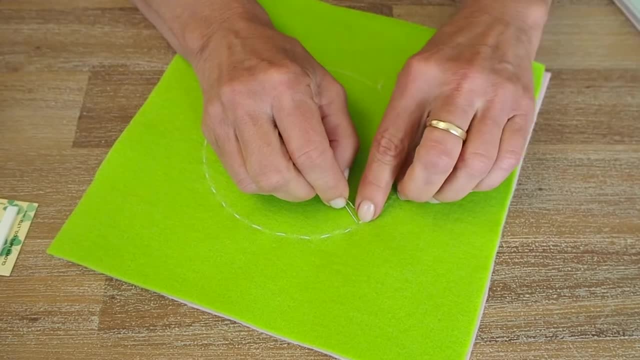 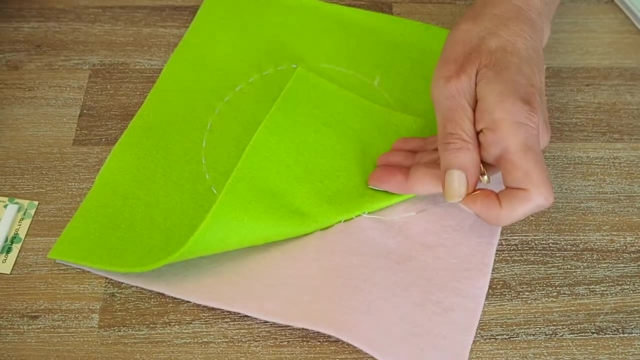 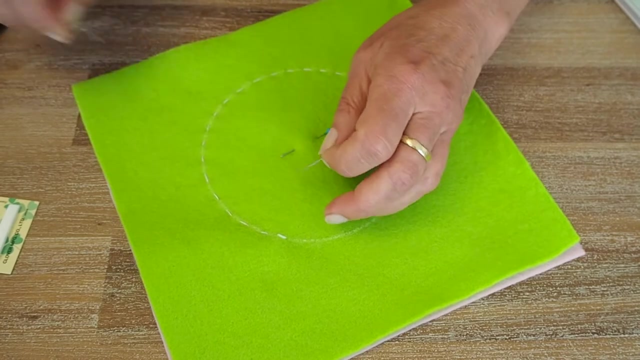 I'm just going to put the needle through that little sort of mark there where the stitch is, and I'm going to push it in between the two layers of felt and that hides the thread. and there we go. now we're going to need to thread our needle again. 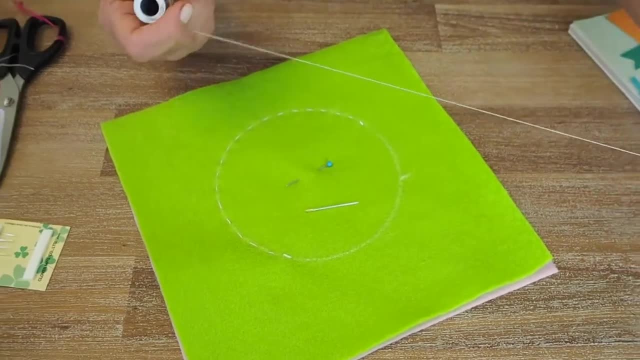 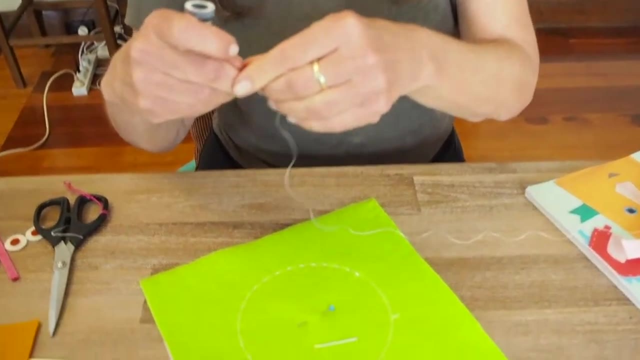 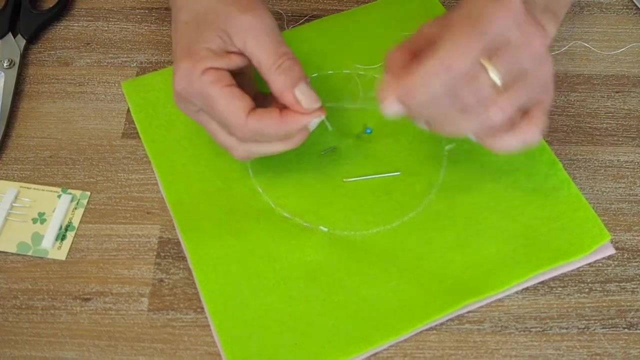 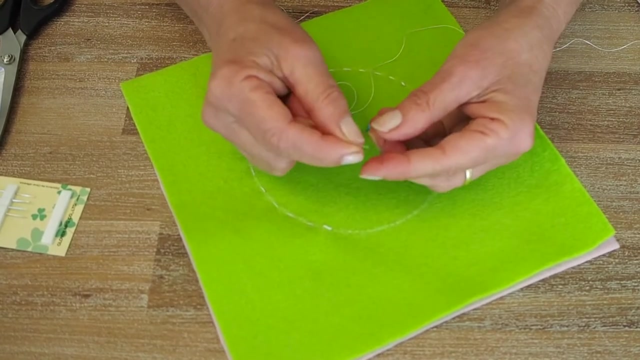 so I'm just going to do exactly so. I'm just going to take it, the thread, pull it out, take it to my shoulder and snip. there's a really nice little method where I put to thread it, where I put the thread through a little piece of paper. but I seem to have lost my paper, so it doesn't matter. 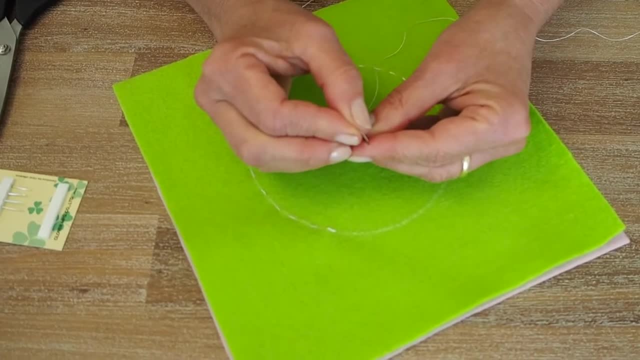 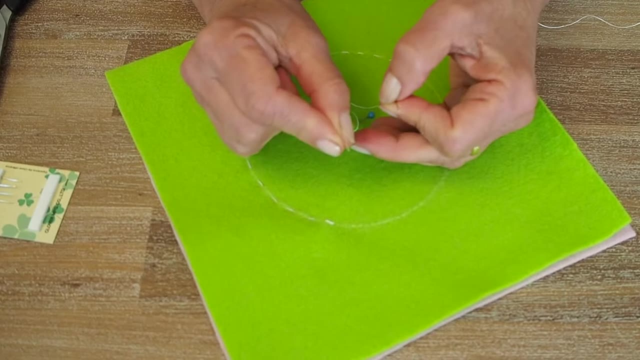 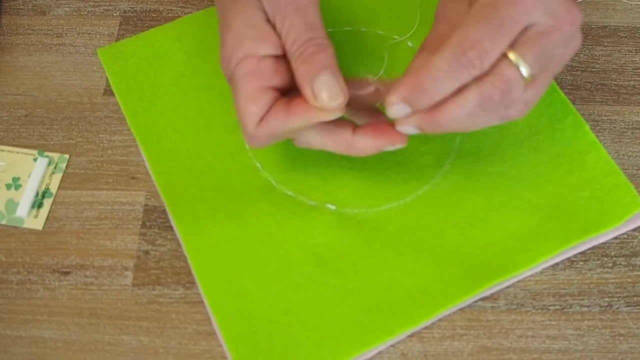 it's uh, you'll find that on my um youtube tutorial, um about threading a needle, and. but I'll show you again when you do the little thread. just you don't want a long bit of thread popping out, just a tiny bit makes it easier, and straight through the needle you're going to bring the two ends together. 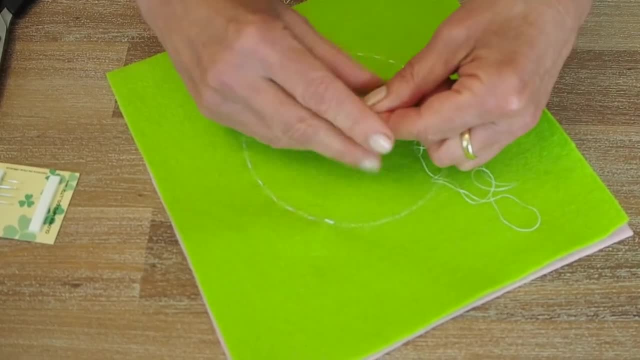 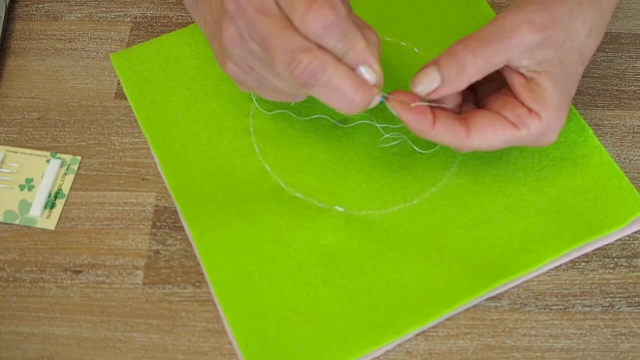 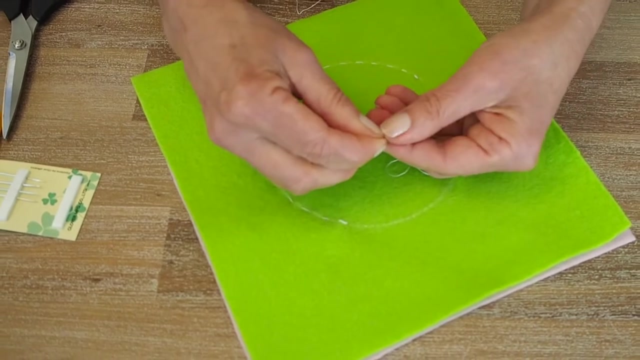 there are my two ends. yep, and I'm just going to show that other way, the same way that I knotted it: the eye of the needle between your thumb and forefinger. get the two ends of the thread, put them in the same place and we're going to start a couple of wraps: one. 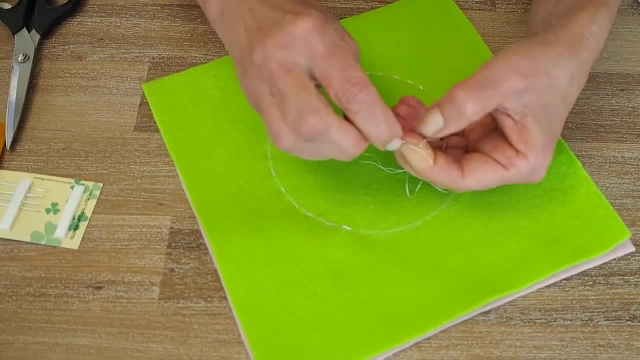 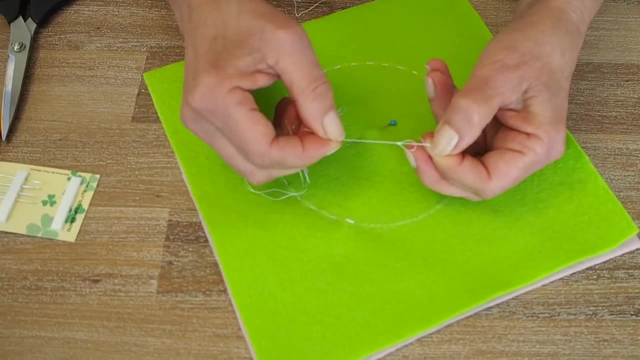 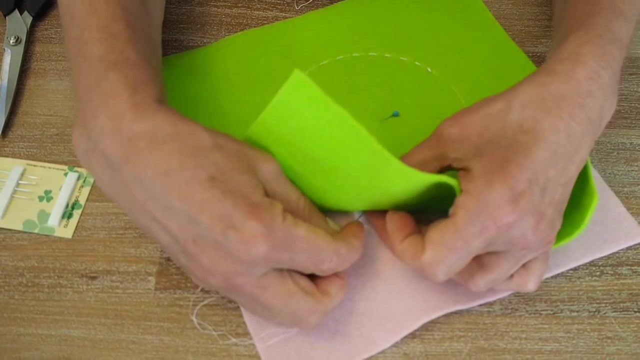 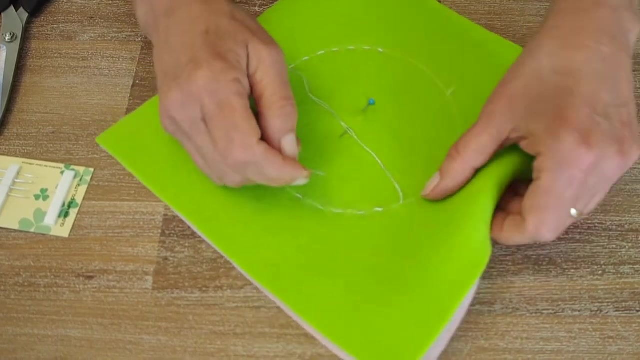 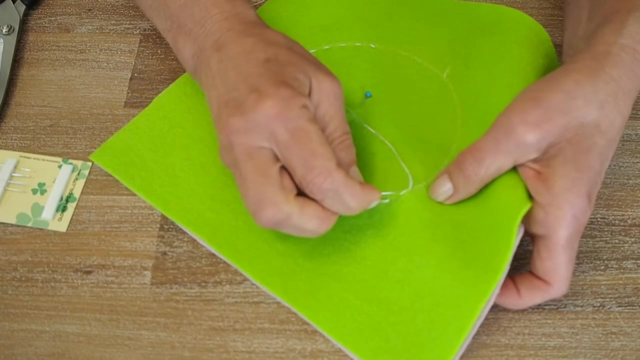 two, three, four and now you're just going to very carefully pull the wraps to the end and there we have our knot again. okay, to start, I'm going to go through the two layers of felt. again needle comes up. remember, we always end and start with a double stitch. so I'm going to go backwards and forwards and I'm going to do this exactly the 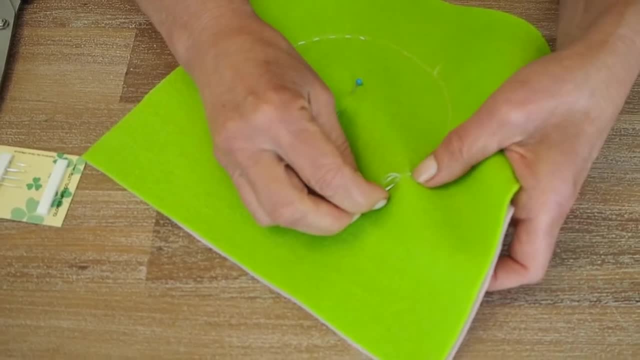 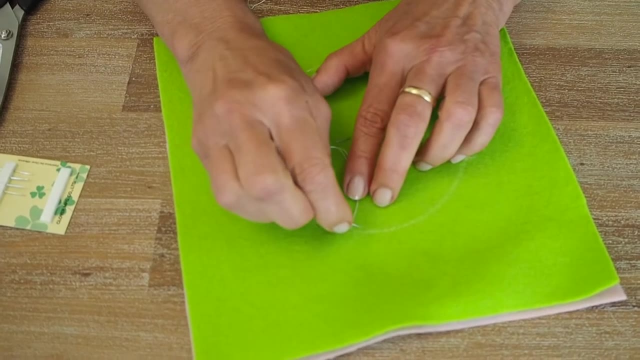 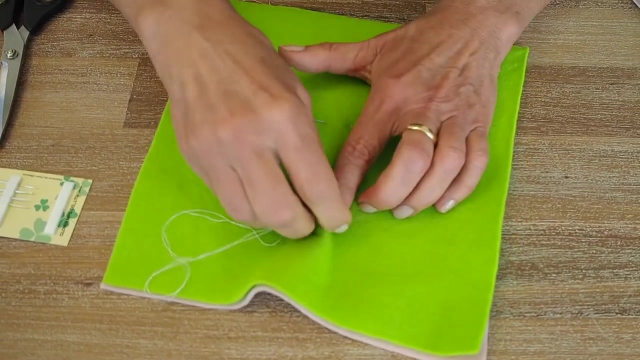 same again, and this time I'm just going to take my needle a little bit further along the line so that you can start your sewing, and this line is great for kids to sew on because they know exactly where they're going. don't forget, if you're joining the global kids sewing party, to send me lots of photos or videos. 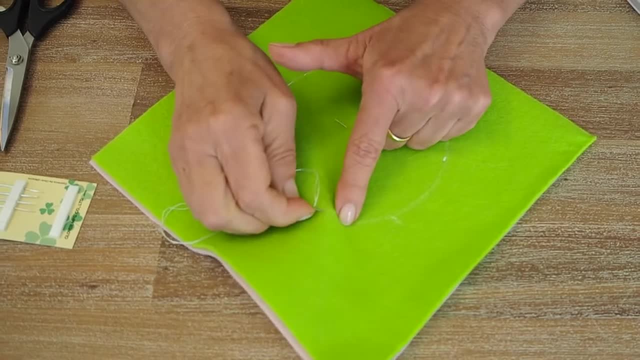 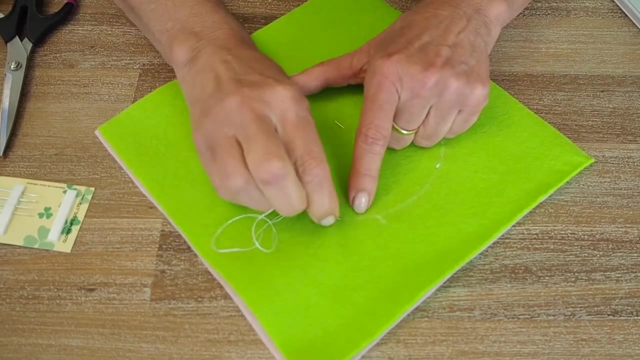 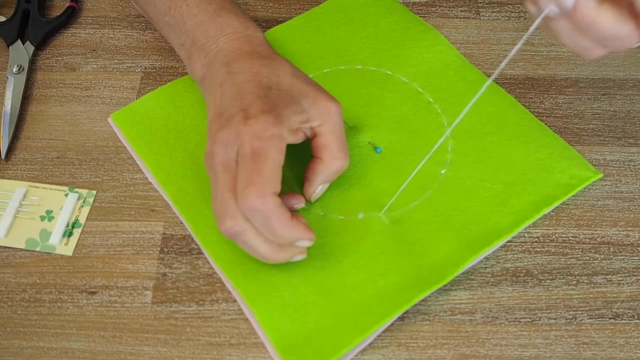 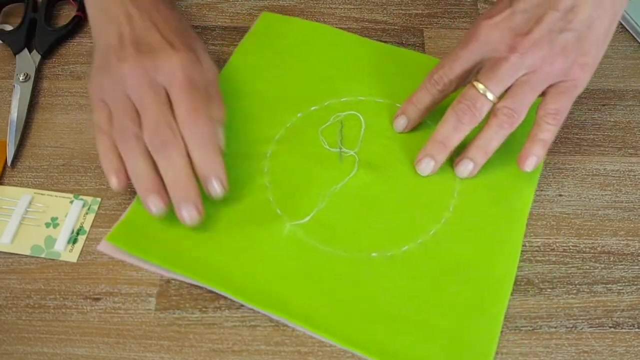 of what your kids are sewing. okay, now we're getting really close to when we have to stuff, so okay, just do it here now. I hope I remembered everything, so now I'm just going to leave, I can take my pin out, because you don't need it anymore, and I've got my circle and my sewing line now. 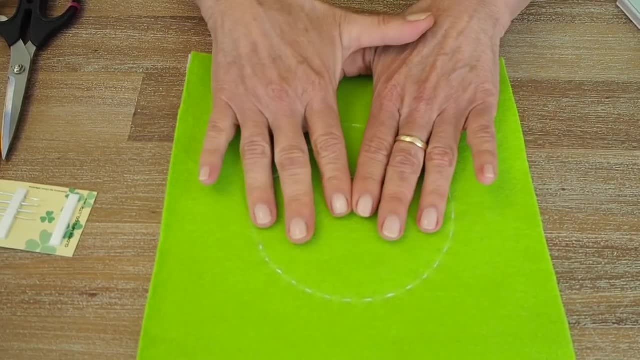 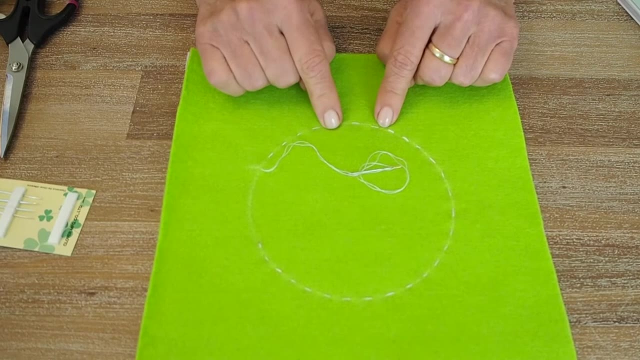 at this point again, you could add your facial features now, but I'm going to leave mine to the end. but before I stuff it, I want to draw on her arms and legs. so, as you can see, this little girl has long arms, and here's her hair. 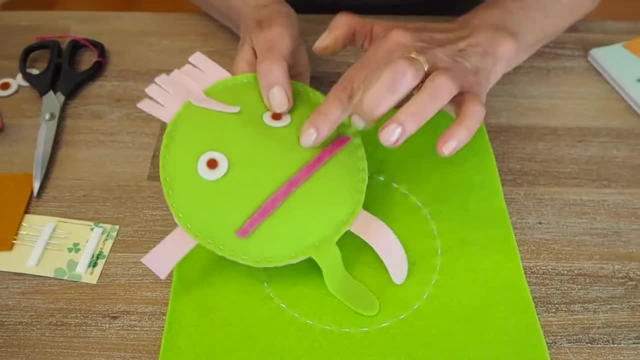 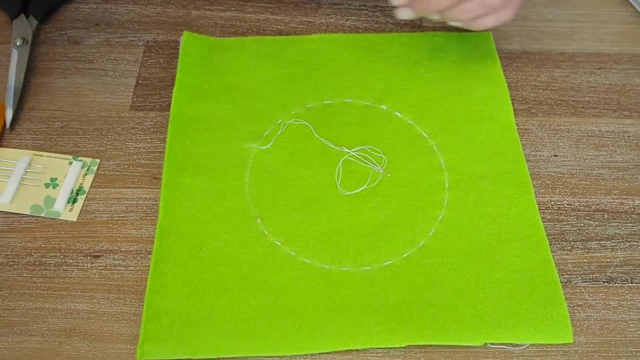 I'm gonna draw on them on. i'm going to make a little baby one for her. so i'm going to- uh, where's my ruler? here we go. so i want her to have hair at the top. i'm just going to draw the lines. no, that's not. 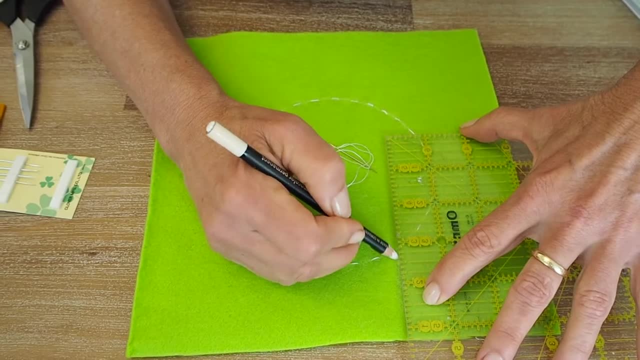 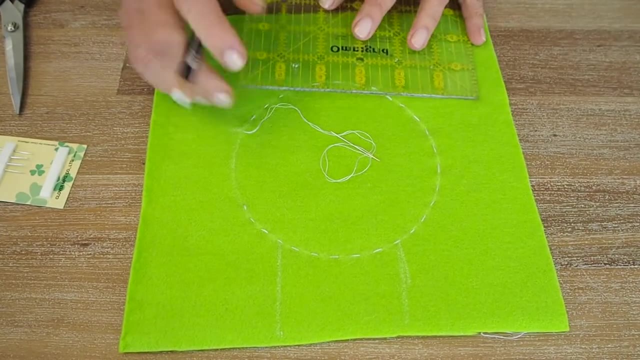 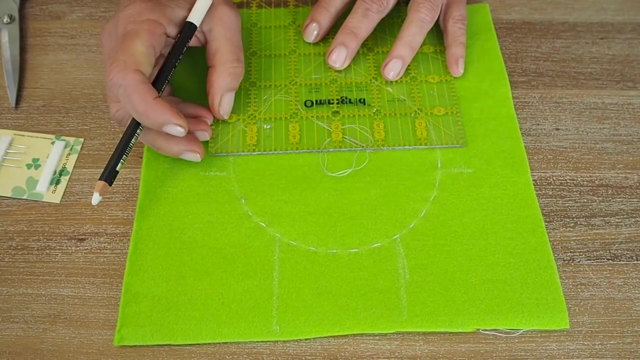 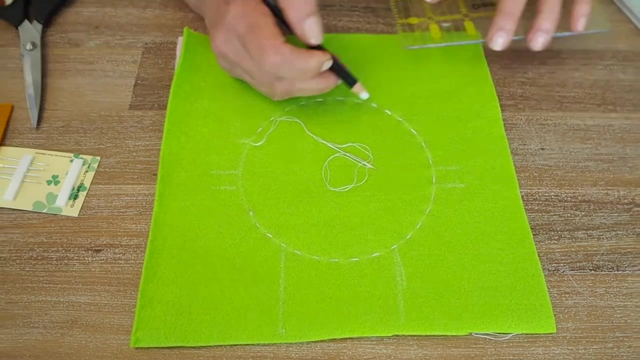 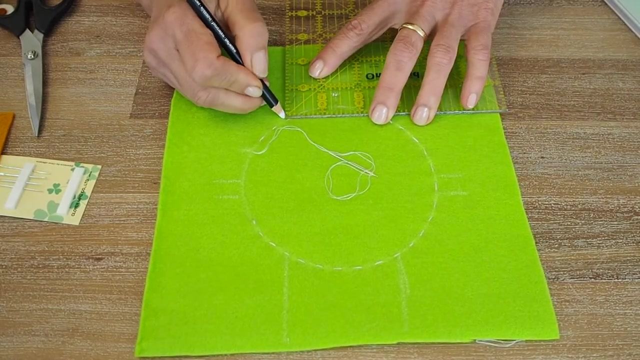 very straight. i'll do line there and it's about there. that should be right. yep, now her arms are going to go around here, so i'm just going to draw lines there and there and i'm going to put her legs here and about here. oh, actually, do that a bit, why? let me just see. i think i should do. 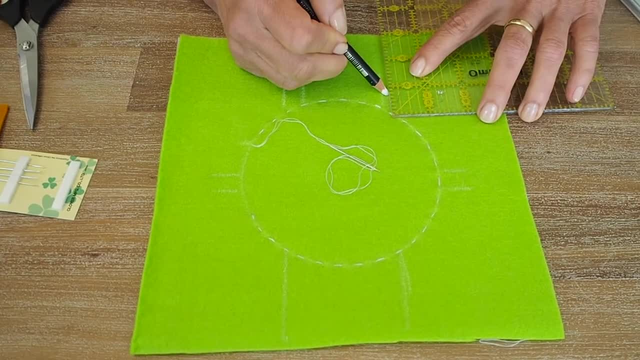 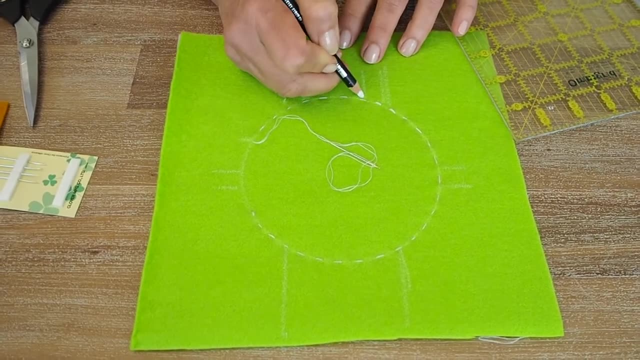 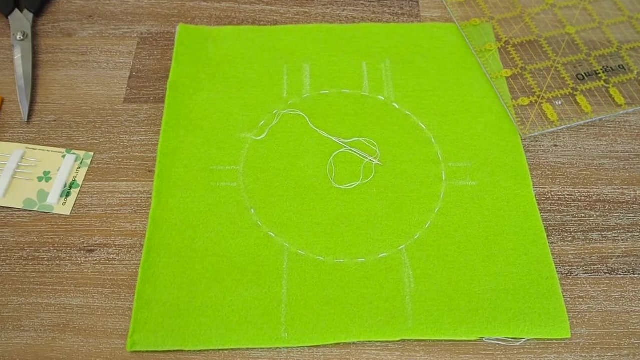 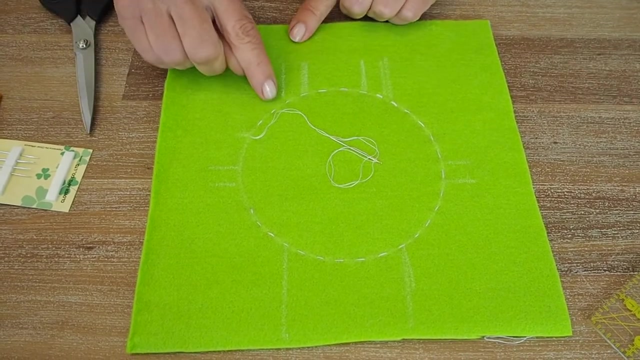 comes out: okay, this is going to do a bit further over and okay, something like that. you can. your kids will know what they want to do, more or less. they're probably better than me designing their senkis, okay. so now i want to cut it out and i'm just going to start cutting around when you cut. 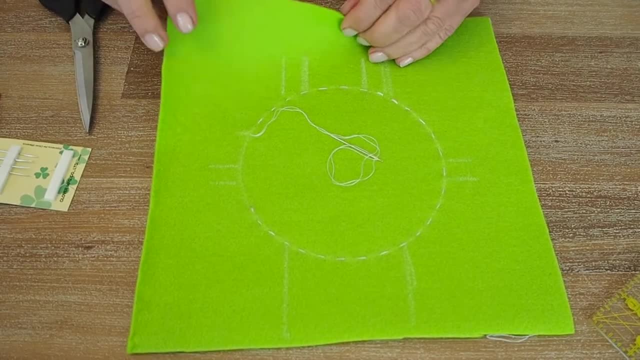 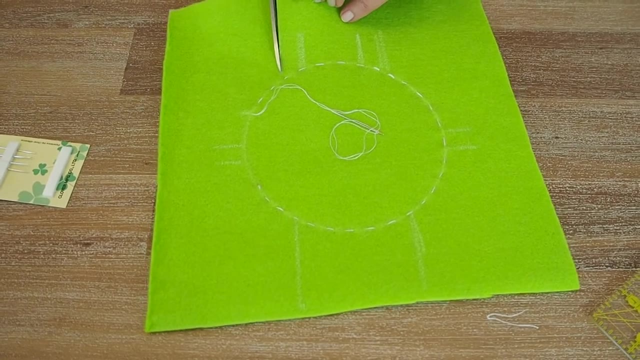 around the stone line, you'll see you leave about a quarter of an inch. now this is pretty thick felt, um, because it's wool felt, so you might have, um, thinner felt, which is probably better for the kids. i guess i'm going to cut the leg out now. you want to make sure your needle is is. 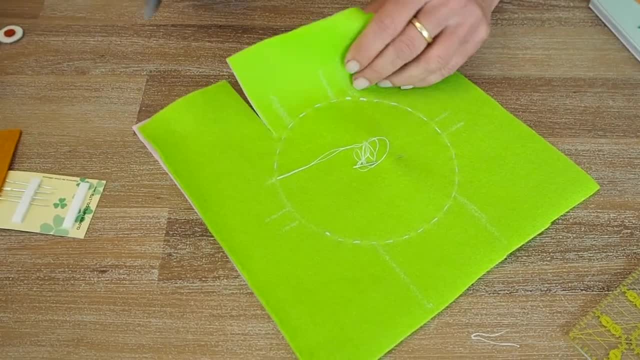 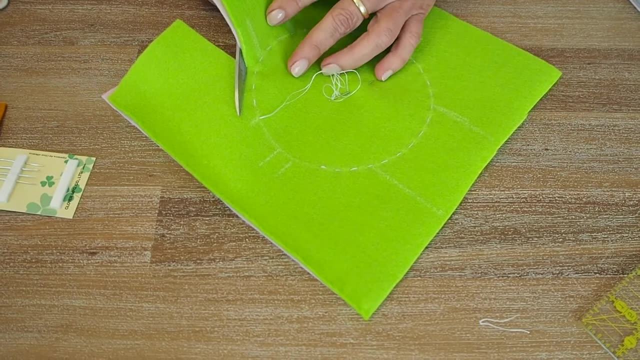 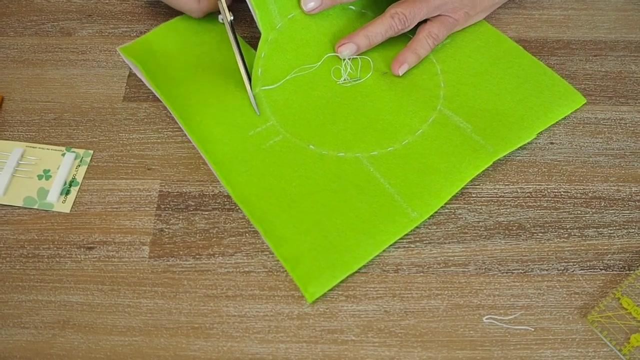 far away from your scissors so you don't want to cut the thread. so now i'm just going to cut. now, remember, i'm cutting around, you know, quarter of an inch ish around the sewing line, and there's my arms up there. okay, great, i'm just going to cut from here. 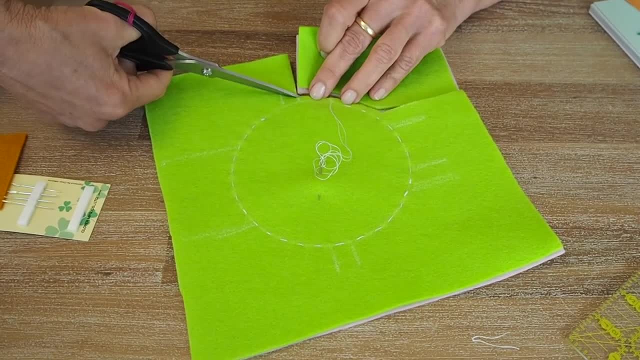 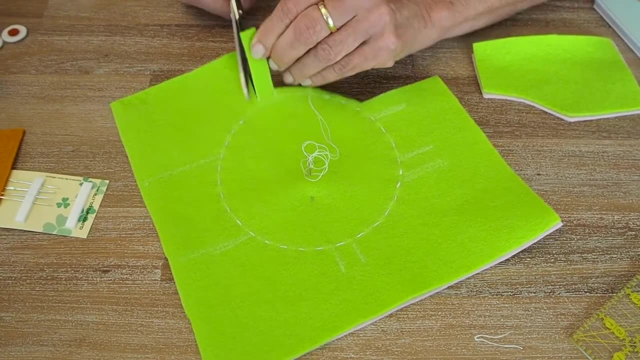 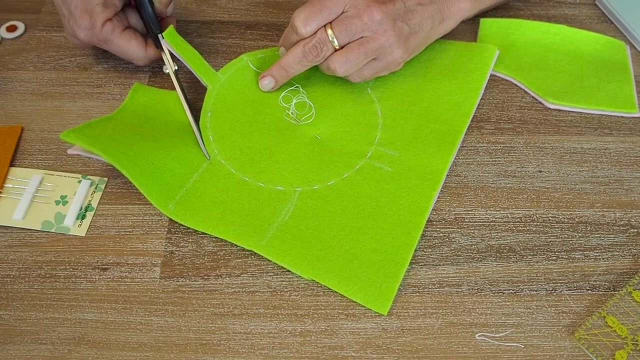 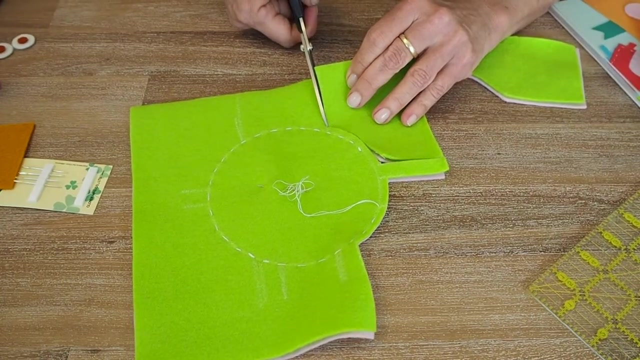 oops, daisy. kids are usually much better, i think, at designing zinkies than than adults. i always get the kids in my classes and my own kids to decide what i want to do. yeah, so them for me, because I think they do a much better job. I never interfere with. 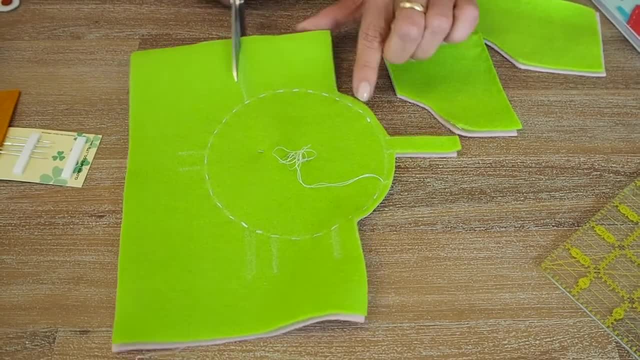 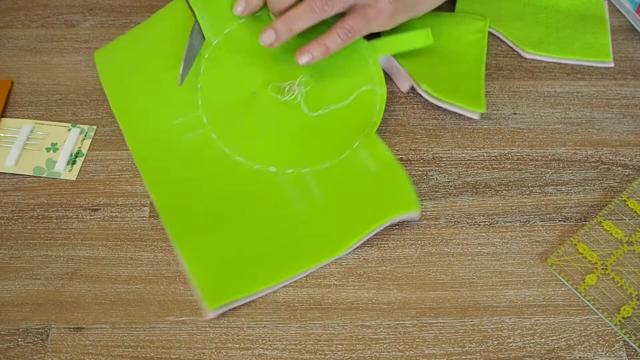 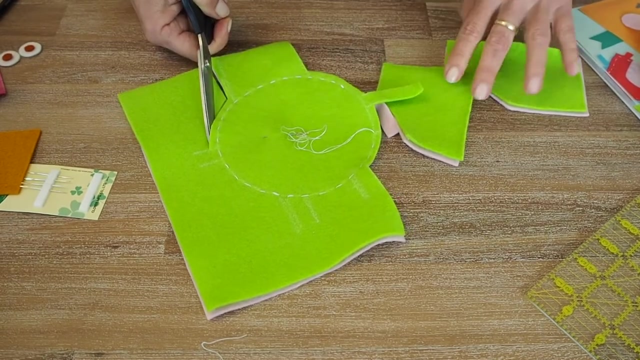 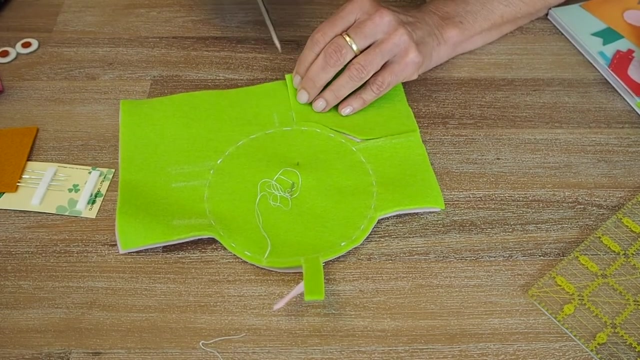 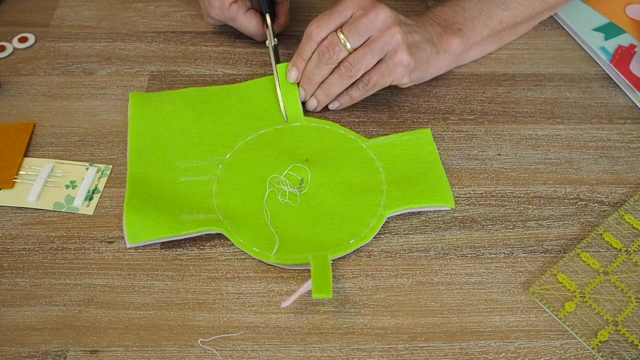 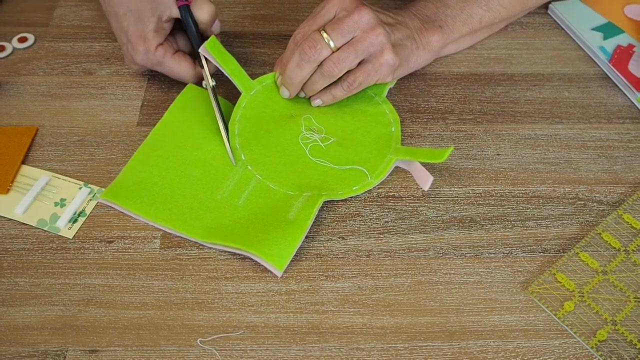 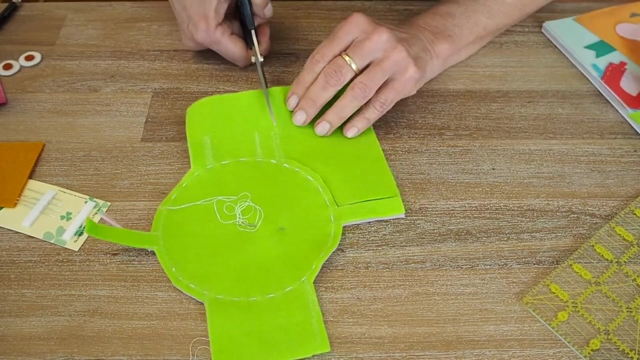 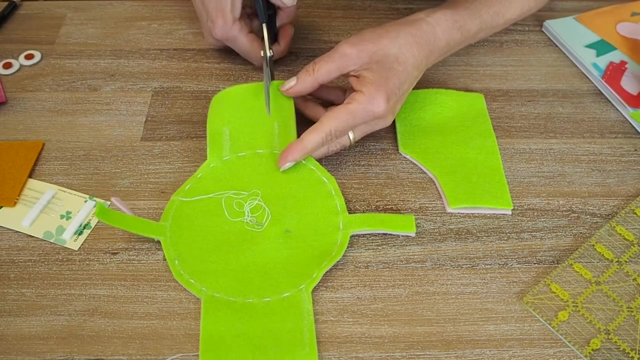 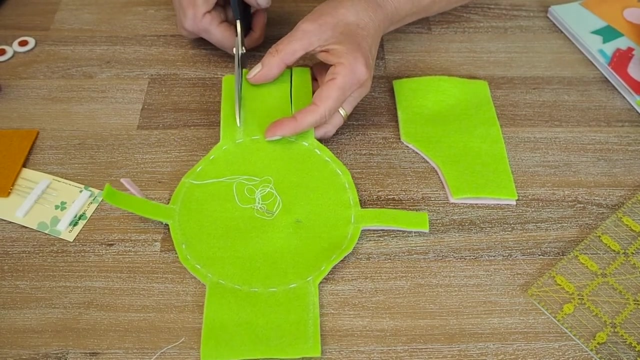 kids creativity because they always do such an amazing job. Okay, that's about right. I'll just do that. cut a bit over there. Okay, remember, about a quarter of an inch away from the sewing line. Oops, Just going to cut her other leg out and then cut in the middle. 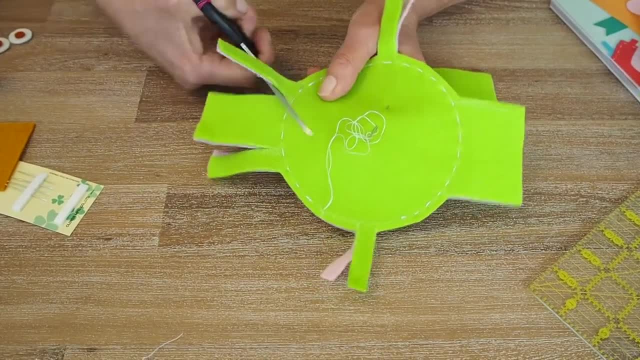 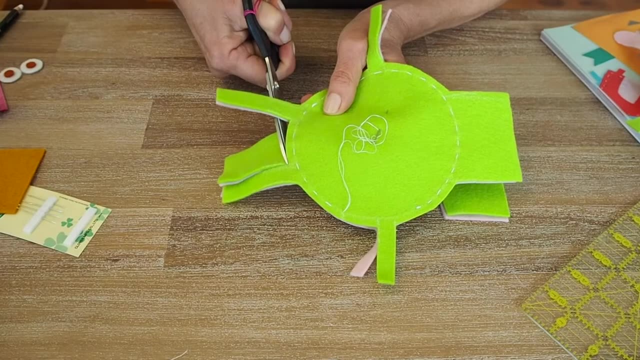 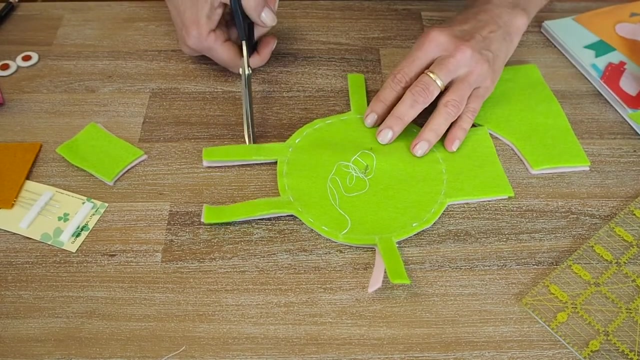 Just turn it around. Okay, so, following the sewing line, I'm just going to cut it out. Now her legs are too long. I want to give her short little arms and legs, so I'm just going to cut the other leg out and then cut in the middle. 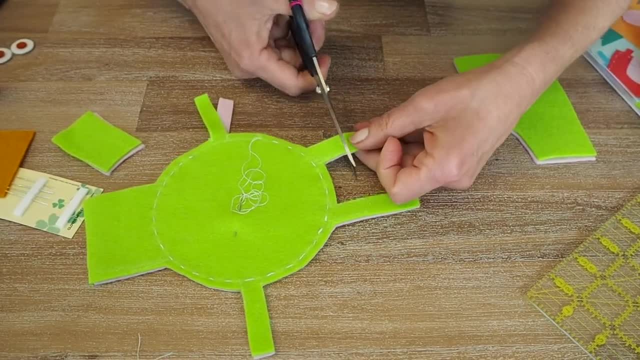 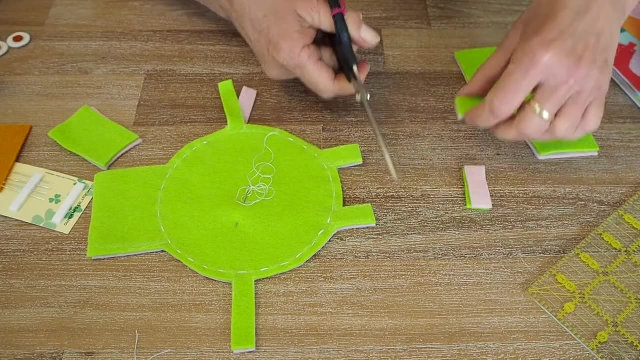 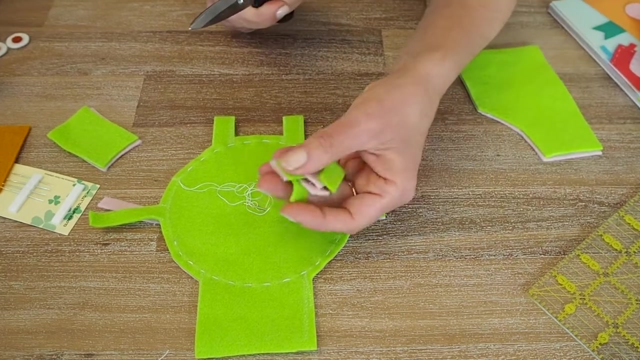 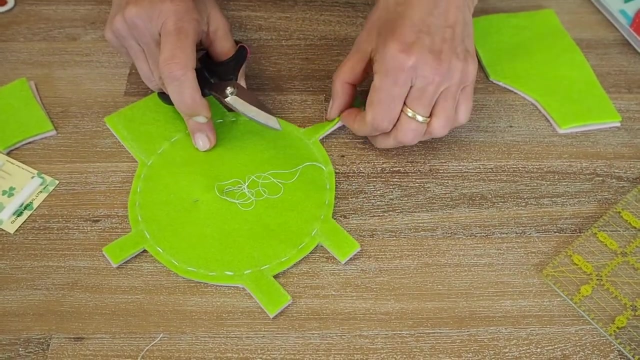 Cut and make her legs a little shorter and cut her arms a little shorter too. These little scraps of felt that I've got left here are really great to keep, because they use them on the facial features. They work really well. Now, as you can see, there's a little bit of a gap between her legs. 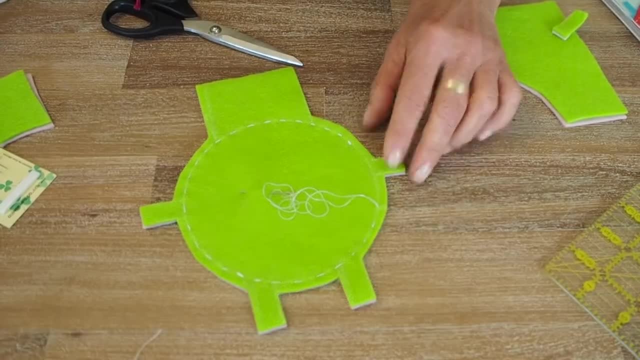 So I'm just going to cut it out and then cut in the middle. Okay so, following the sewing line, I'm just going to cut in the middle. Just following the sewing line, I'm just going to cut in the middle. I've done a little. oh, I'll show you here. 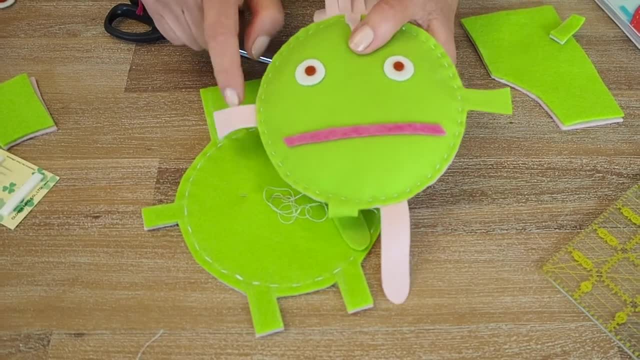 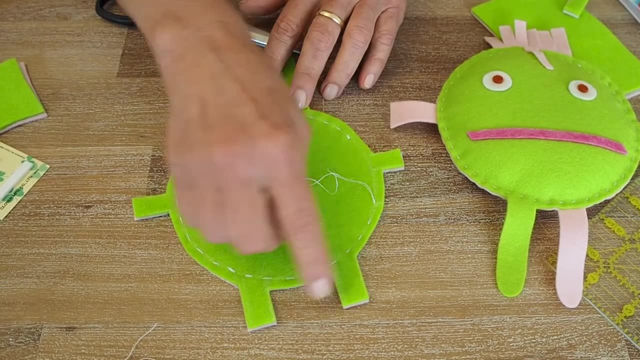 See, this little girl has got a pink arm and a green arm and pink and green legs. so you can actually chop or cut the top layer or bottom layer of either the legs and arms, just to get different effects. So I'm just going to cut the top green layer off. 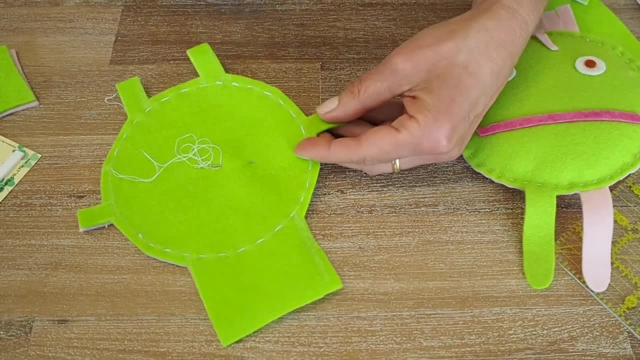 Now make sure that the pink arm is out of the way, and I'm just going to cut the green arm off. Now she's got her little pink arm out. Now I'm going to turn around here and I'm just going to cut the other leg off. 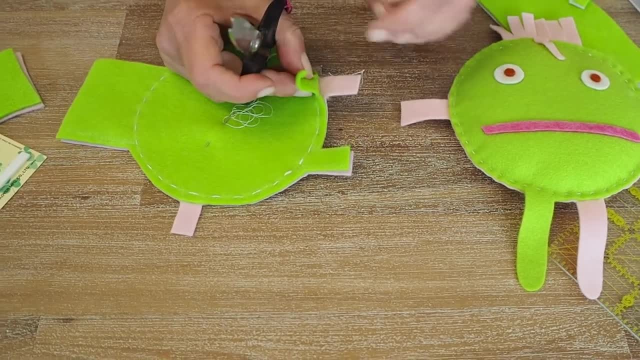 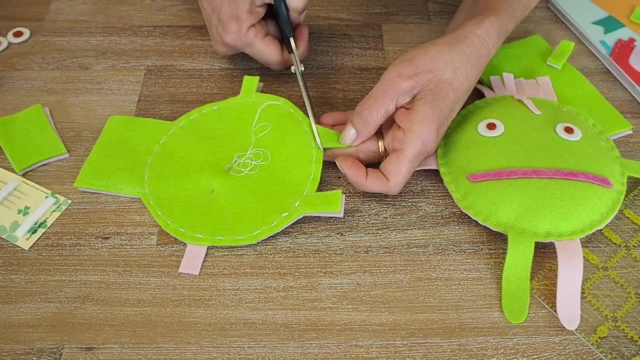 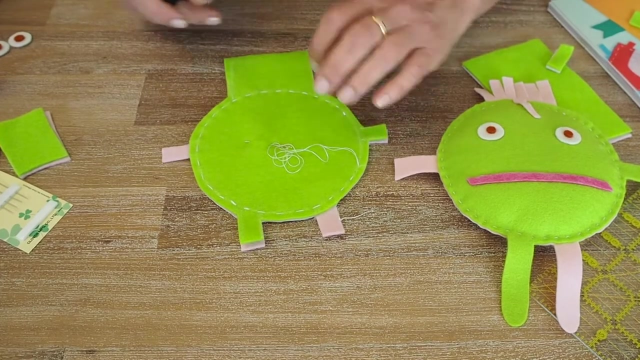 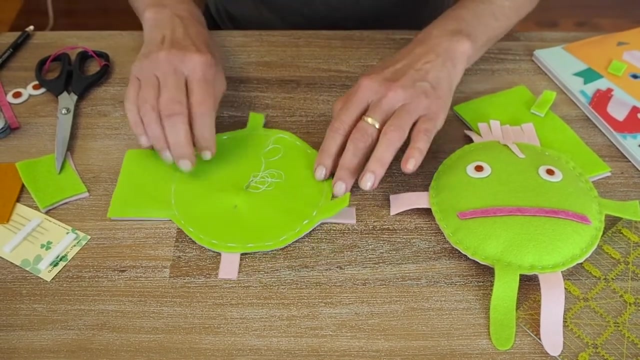 and I'm going to do the same with this leg over here. if you want to flip the pink leg out of the way so you don't cut it off, and there we go. so and if you want, you can take the pink leg off the back if you want, or you can leave it there, it doesn't matter. now, oh, almost forget, I'm gonna give her. 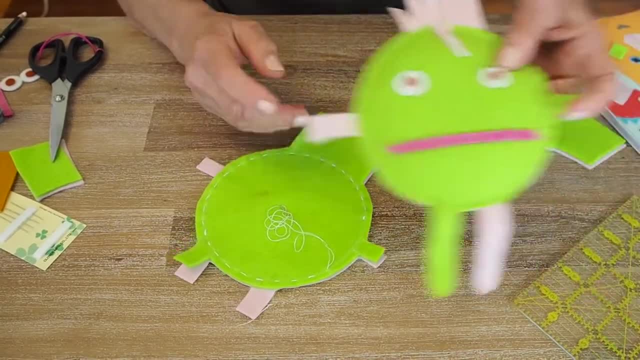 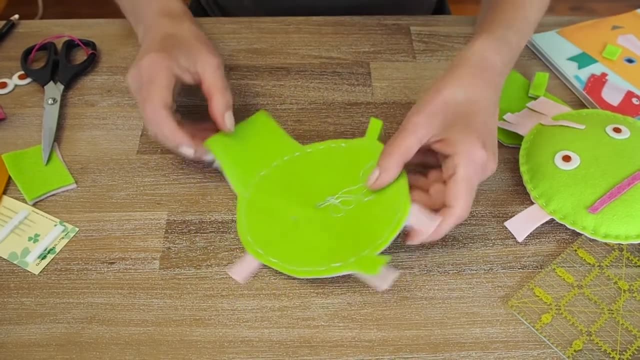 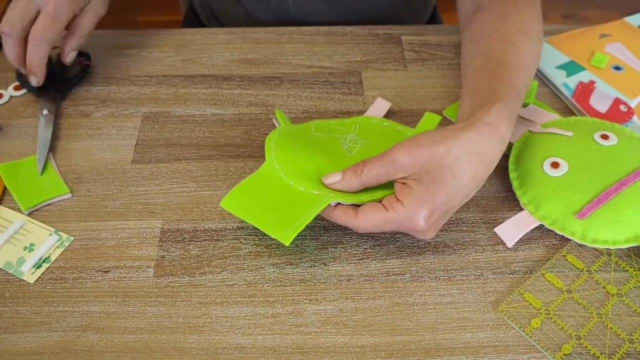 hair. but I'm just gonna, I think I'm going to give her, just like her mum, I'm going to give her pink hair. so, instead of cutting through the two layers, I'm just going to cut the top layer of green off. remember, I'm going to just flip that around and I'm just going to cut the green layer off and 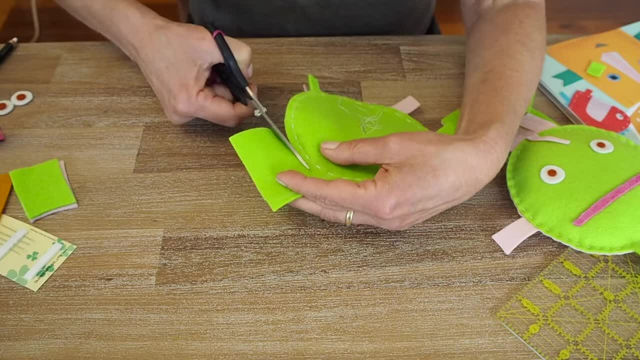 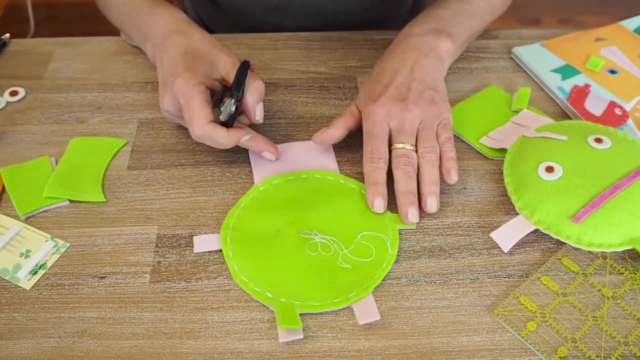 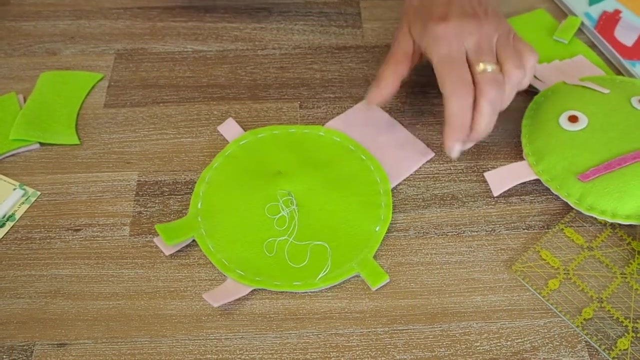 hopefully, hopefully, you can see what I'm doing, okay, so now I've got her pink hair and I'm going to. I want to give her little fringes, so I think I might make her a little bit shorter, because she's only a little baby, so she doesn't really have that. 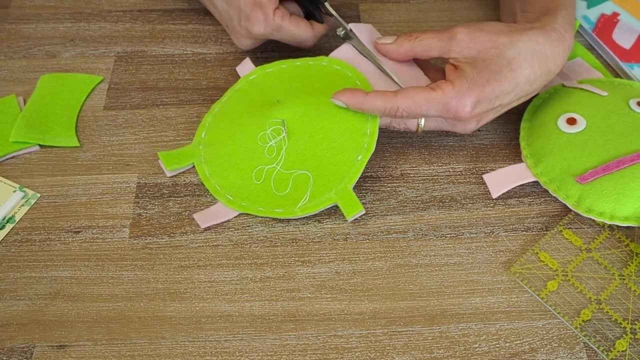 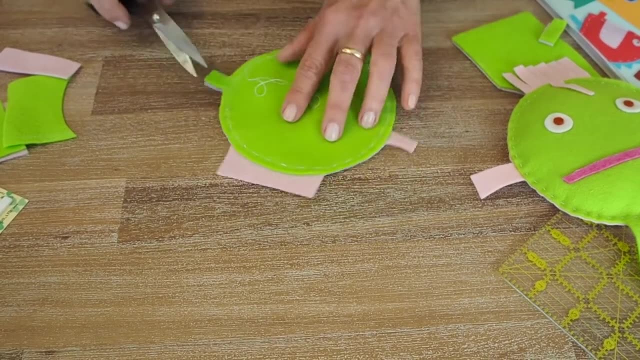 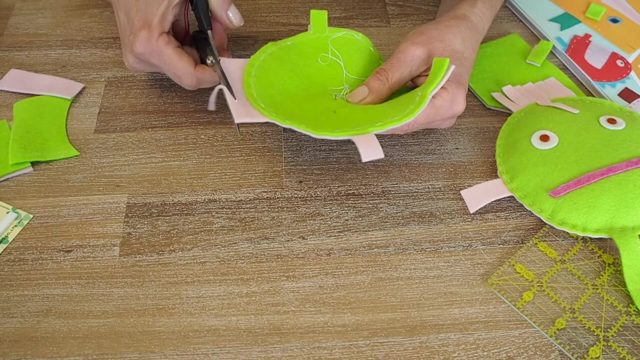 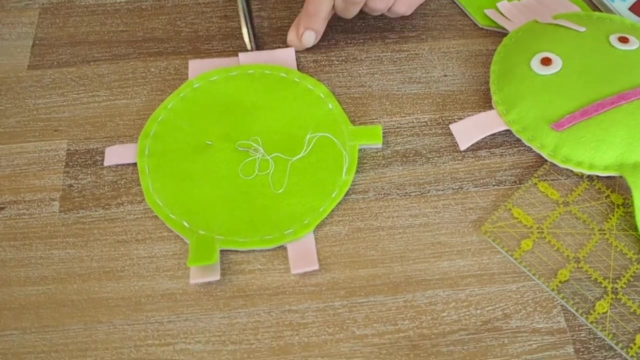 long hair. of course, that's one of the fun things cutting hair. okay, now to cut her hair looks like I haven't cut that straight at the end. I'm just going to cut that straight a little bit, okay, so I'm going to cut one slit in the middle and I'm just going to keep on cutting the middle. 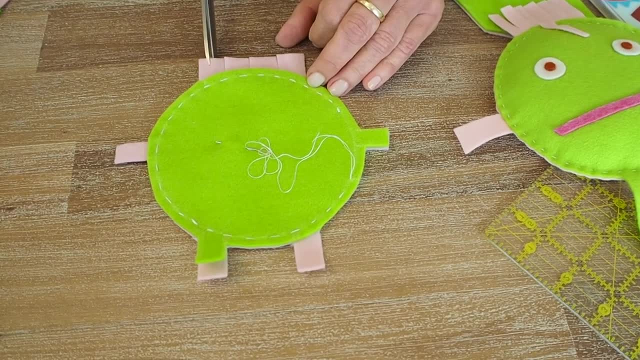 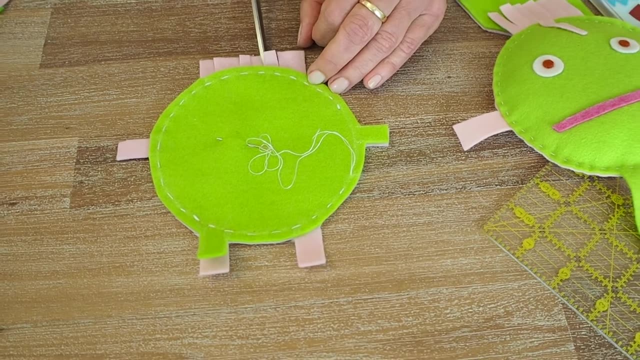 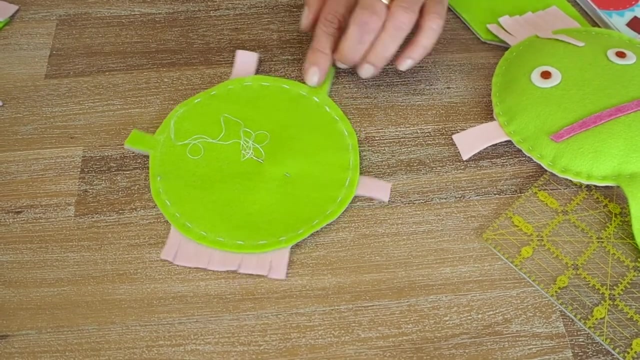 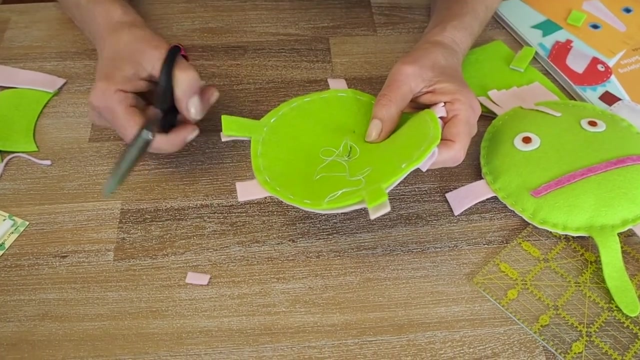 of these two, and now the middle of these two, middle of these two slits, middle and middle. okay, now let's have a look at her. hmm, I think I might make her legs a little shorter. I think they need to be little. so I'm just going to snip there and I'm just going. 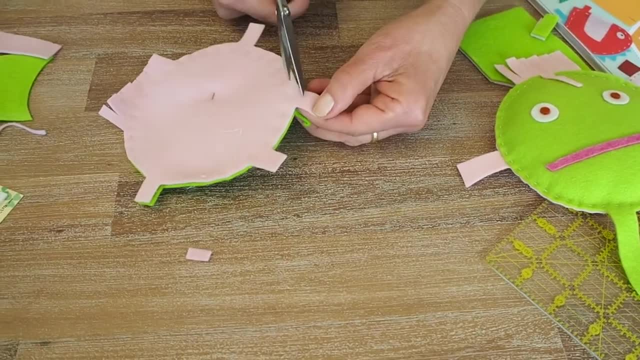 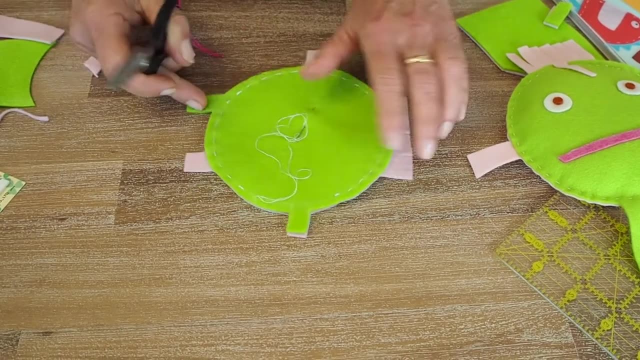 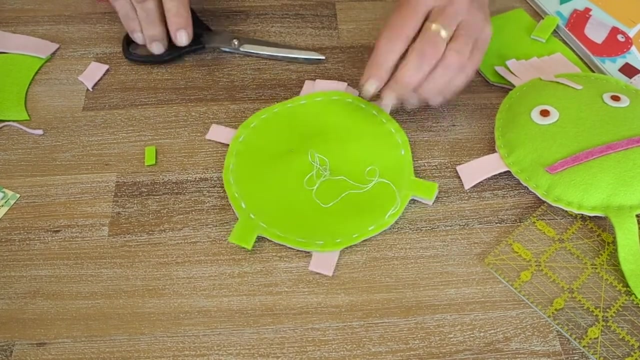 to cut the pink leg off at the back because I don't want that there, but of course you can leave it, so I'm just going to go cut that off, okay, and of course we're going to cut this leg off a little bit to match the other one. and, yeah, I think the arms need to be a bit shorter too. 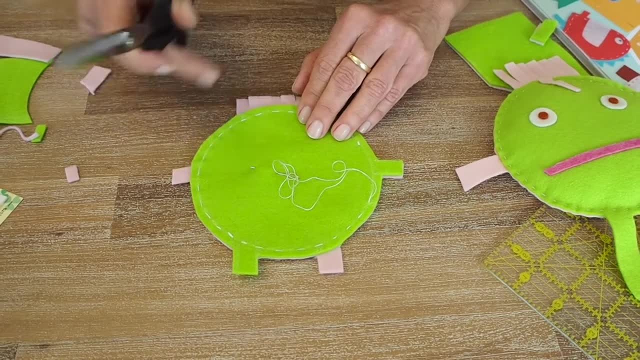 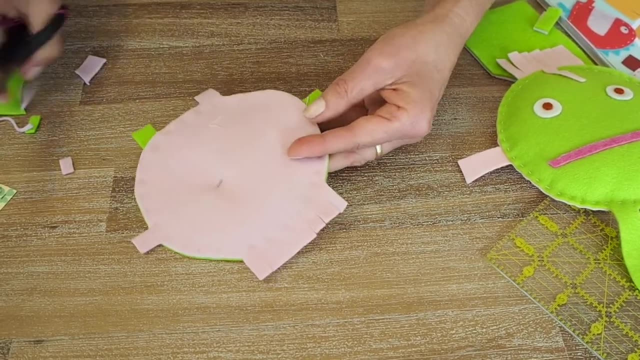 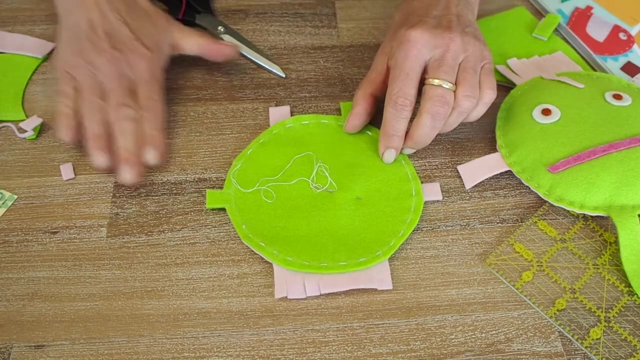 there and I'm going to cut the little arm off the back, the pink one, which we don't want- and of course we want this arm a little shorter too. now I think I've done everything and I think we are now ready to stuff my little girl. 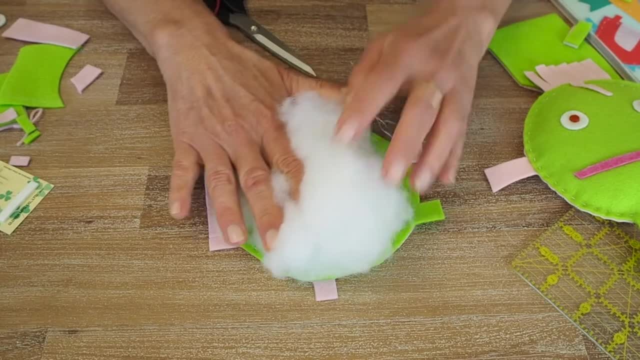 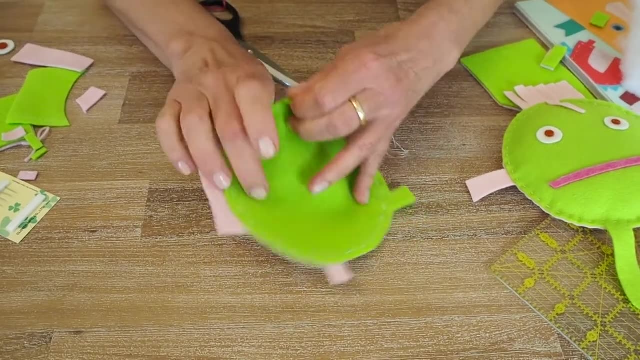 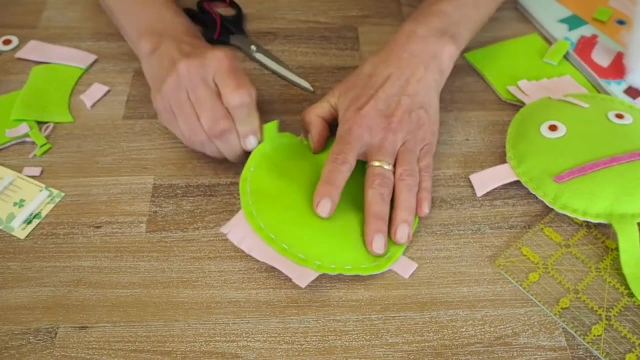 so here's a big water stuffer. you don't want to stuff the whole thing in there because it makes it a bit lumpy. you take little pieces of stuffing, sort of roll it up in your hand and start pushing it through right to the end of your circle. um Zenki, you can use a pencil, if you have, or something just to get it right. 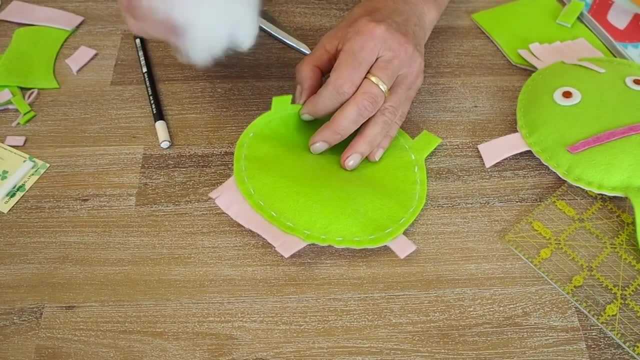 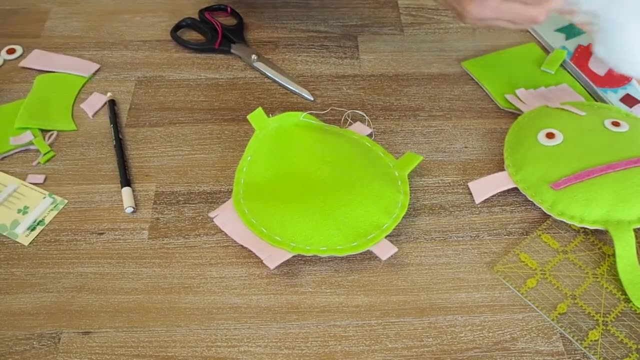 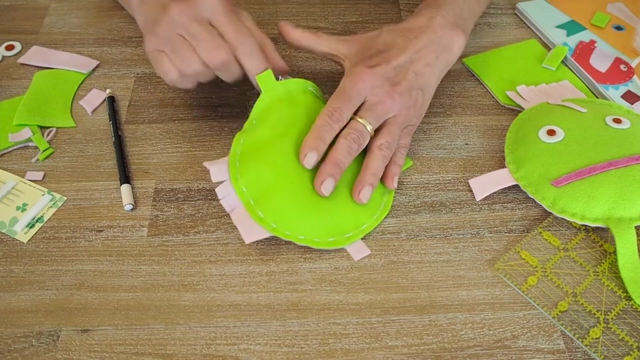 to the ends and you just keep on adding little rolls of balls of stuffing, pushing in with your fingers, pencil, whatever's best for you. oops, and of course, this is um softies or Zenki's favorite part when they get their stuffing, because it makes them feel real. 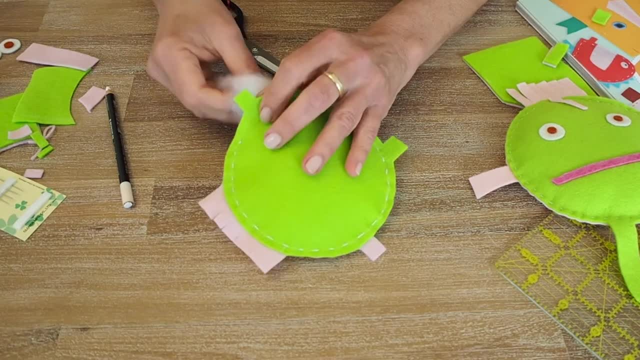 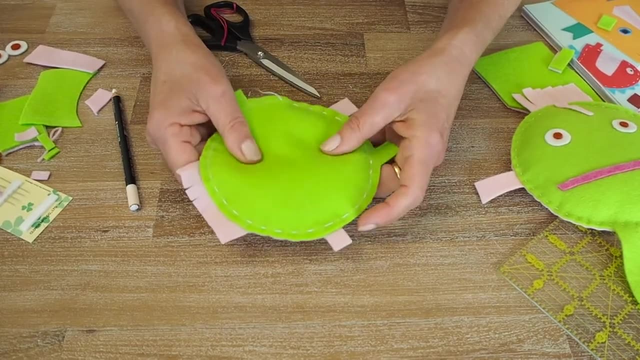 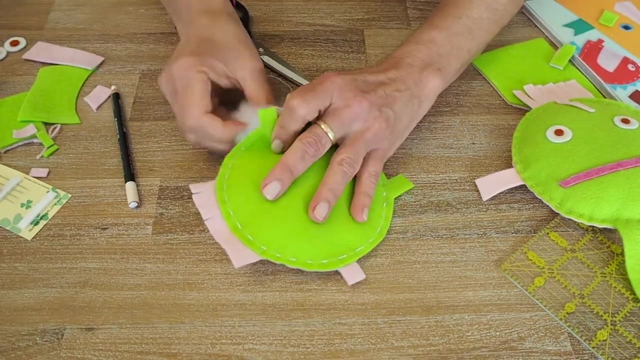 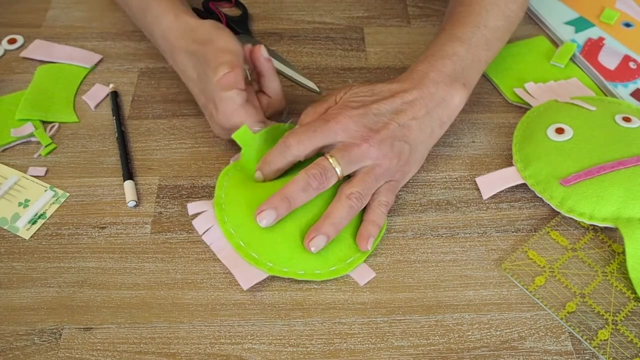 because they are okay. I'm going to add a little bit more, okay. and let's just have a look at her. I think I think she needs just a tiny bit more stuffing, okay, and a little bit down here, okay. I think she's feeling very good now. I'm going to just push the stuffing a little bit. 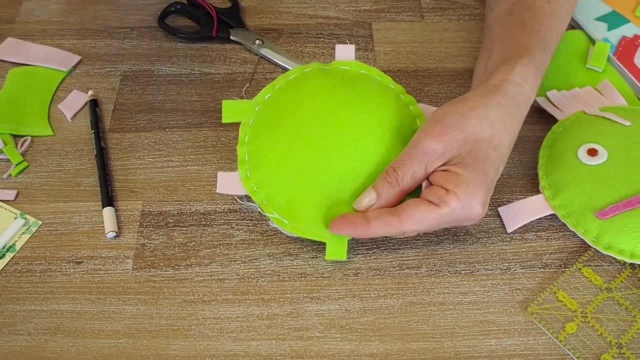 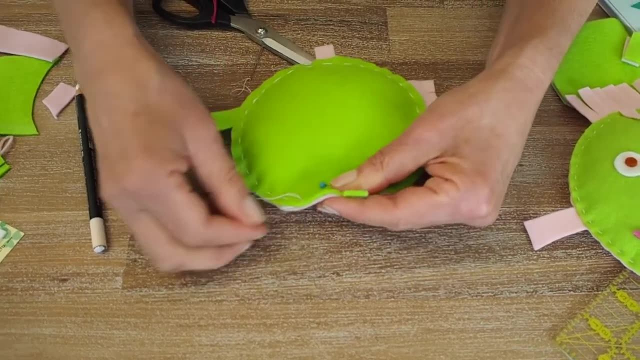 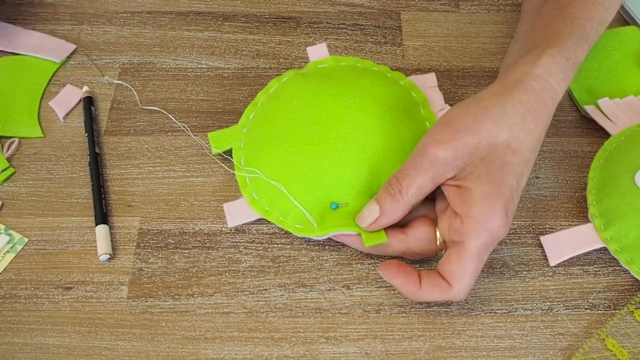 away from that sort of sewing line and I'm going to pin it there to keep the stuffing out of the way while you sew. okay, so you're going to keep on sewing your running Stitches. let's get rid of some of my bits and pieces. so the sewing. 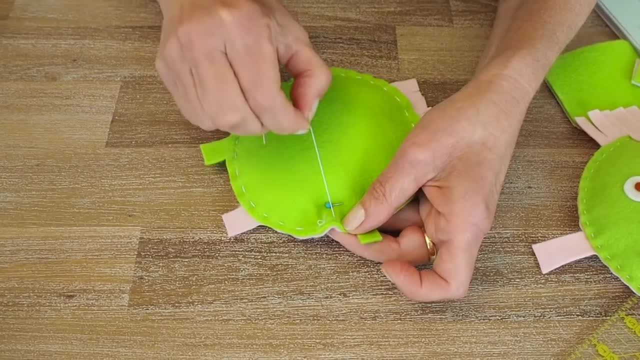 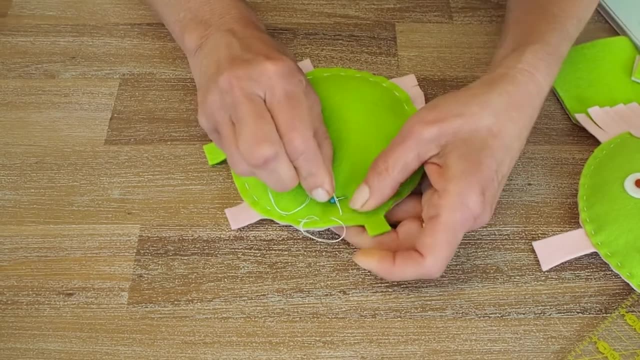 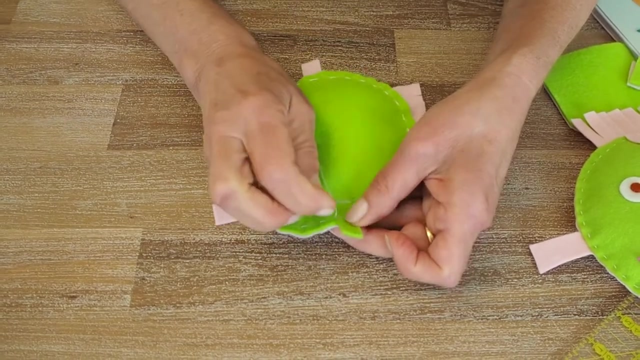 up down. if your thread tangles, just give it a little pull. it does that sometimes because it's just been on a roll for too long. there we go. okay, there's your line there. so in case you can't see it, you can either draw the line again. 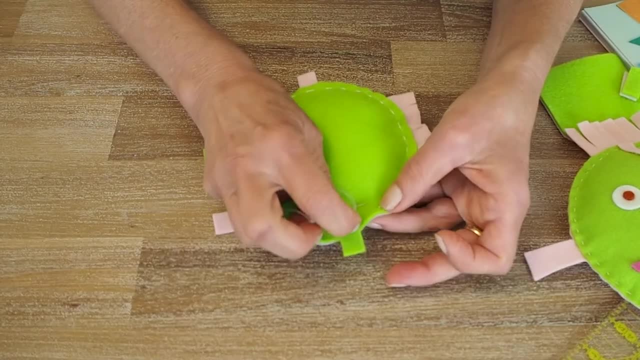 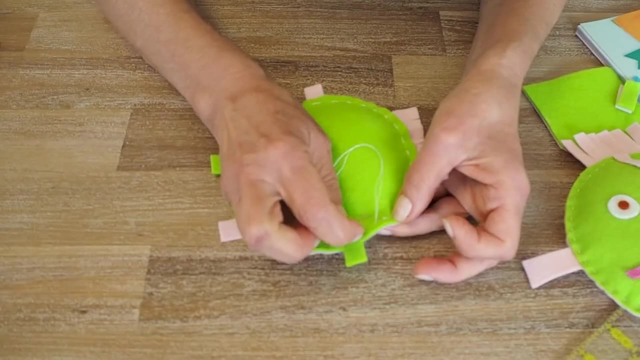 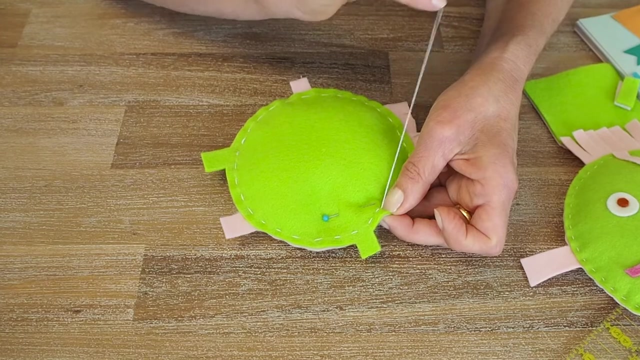 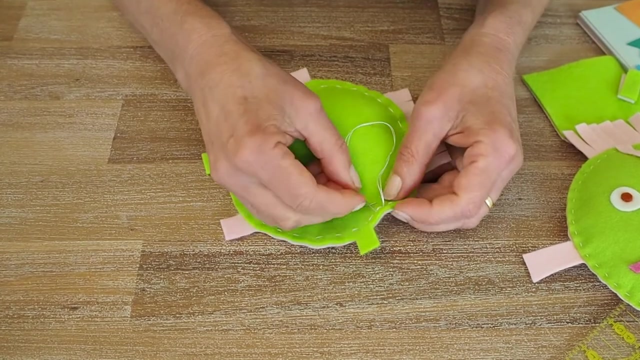 or just draw the line with your needle. okay, so now I've got my last Stitch and I'm going to do my back Stitch. I've got to go backwards and forwards, again backwards and forwards and I'm going to take the needle through that last little place where you put the. 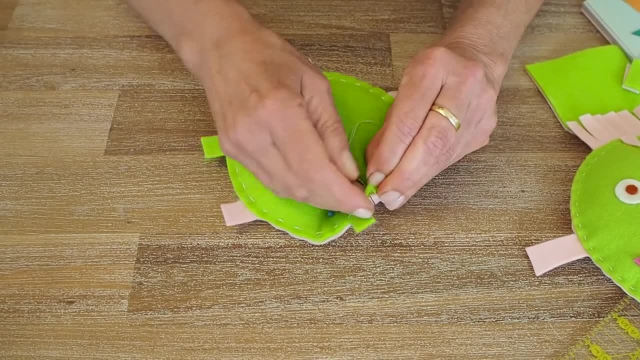 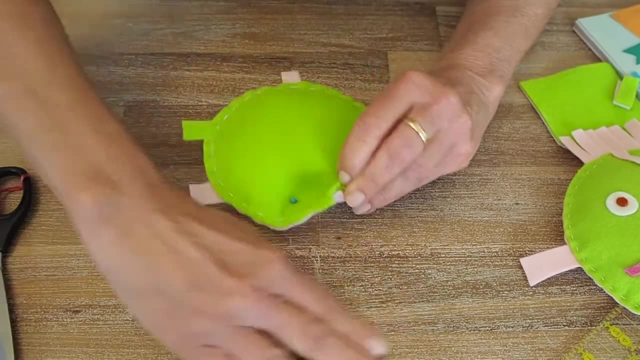 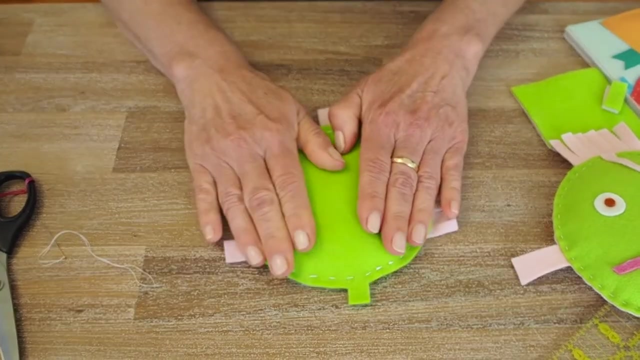 needle and I'm going to take it between the two layers of felt and I'm going to carefully snip it and I'm going to take my pinner and give her a little shake just to make sure that the stuffing gets everywhere. and now I'm ready to um what I'm ready to put on her facial features. so 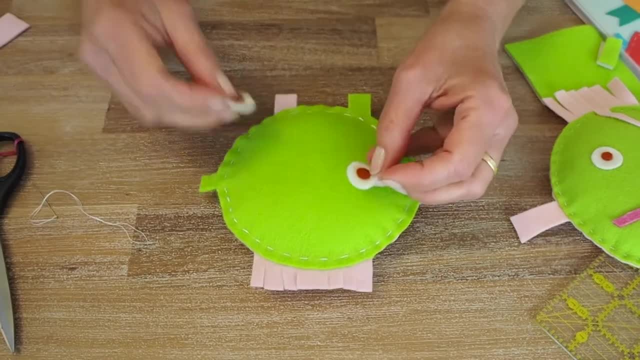 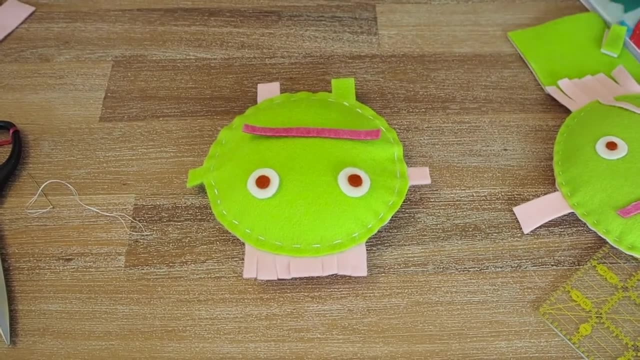 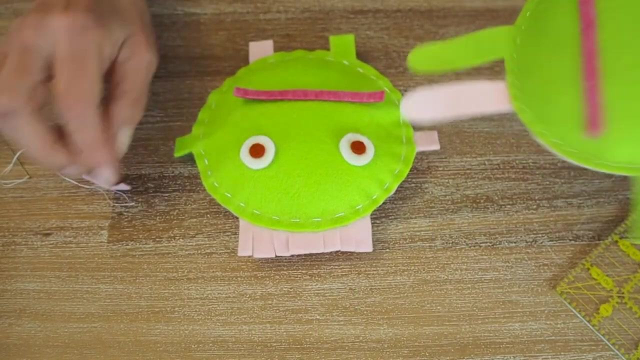 I've already got some bits cut out. I've got two little eyes. I've glued the pupils on and I've got a mouth for her and, of course, because she wants to look just like her mom- sorry, I'm going to give her this little lock. okay, so I've got my glue gun. oh, I did forget to tell you about glues. now. 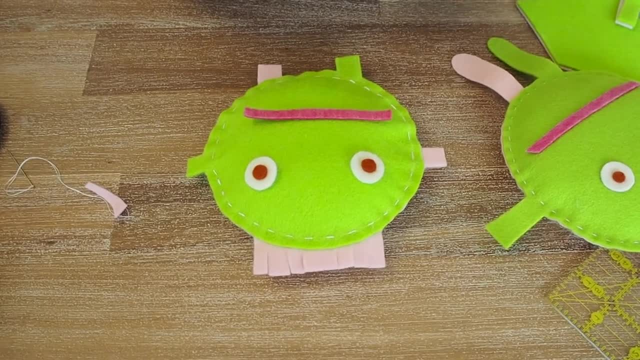 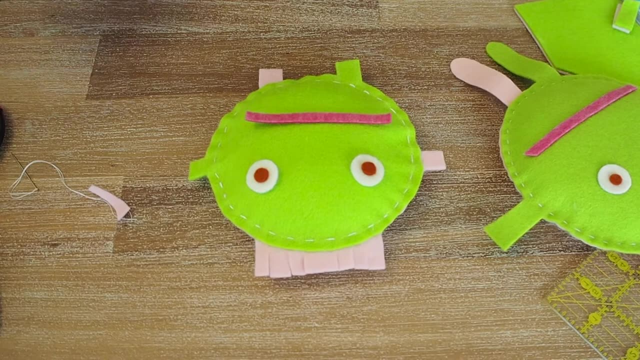 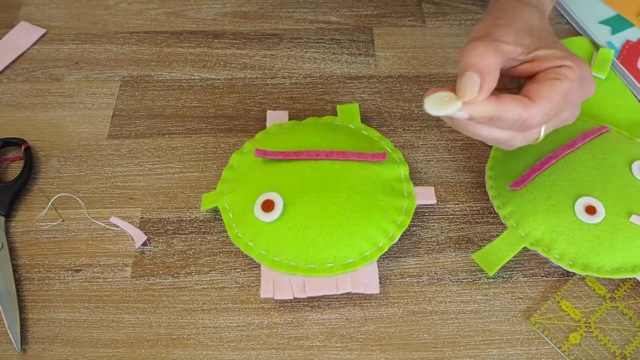 glues can be a little bit um tricky when you're working with felt. some of the fabric glues don't work on felt, so it's a little bit of testing to see what works um to glue. so I'm just using a glue gun today. so I'm just going to a little glue and let's put the first eye on I'm going to put it there. 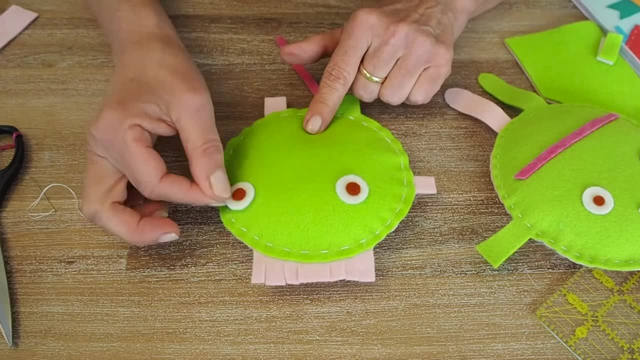 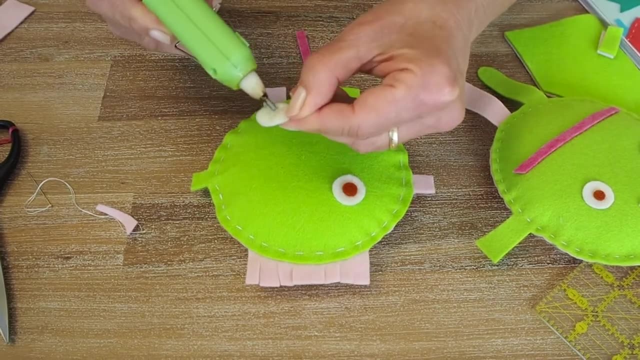 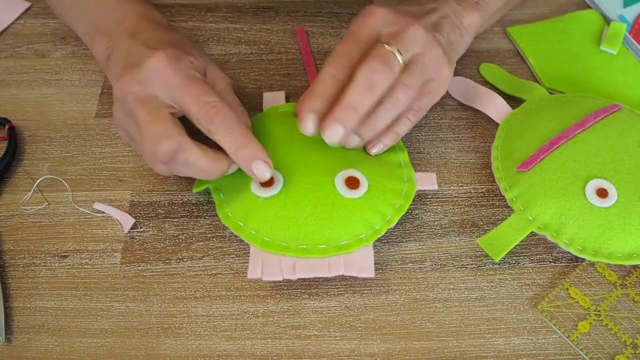 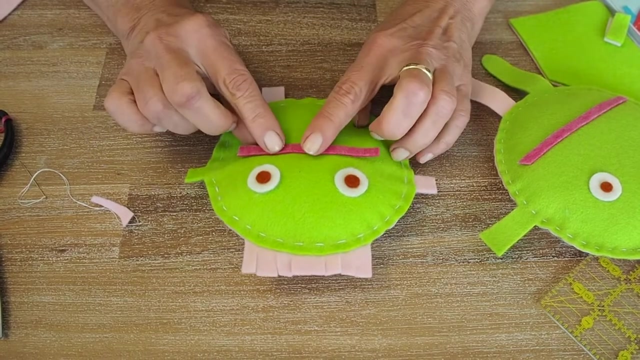 and you can test, you know, having the eyes closer or further and see what you like. I think I like her eye about there, so I'm going to get a bit more glue. oh, you can see my cat, hear my cat in the background. okay, and I've got her mouth, of course. you know you can sort of play around before you glue on. 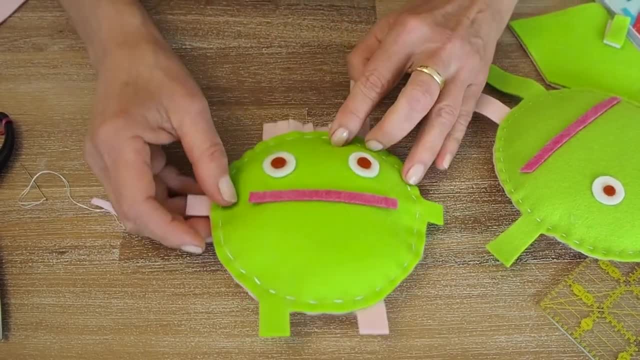 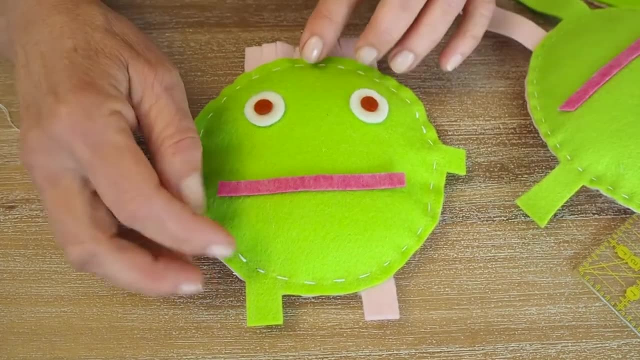 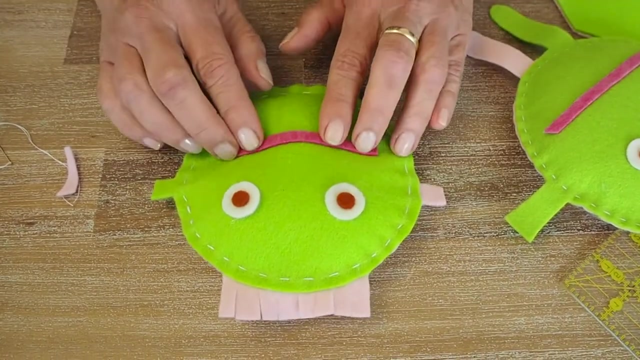 you know, do you like it further up? I'll just turn her around so you can see her perhaps better. you can see her mouth further up down in the middle, longer, shorter. just play around and see whatever you like, so I'm just going to put her mouth about. I think it looks good there, so I'm going to get.